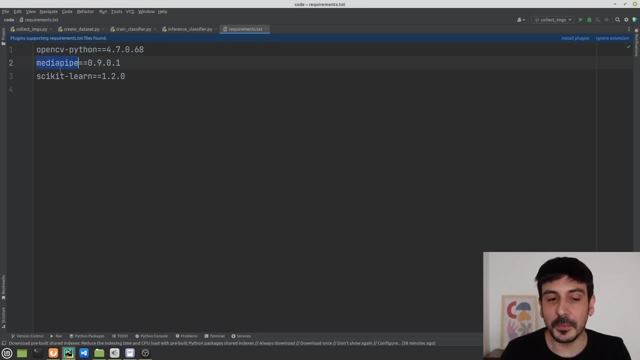 starting with this tutorial, We are going to work with OpenCV MediaPipe. This is a very important library we are going to use today, And we are also going to work with CKIT Learn. So these are the requirements for today's tutorial, And now let me tell you about the 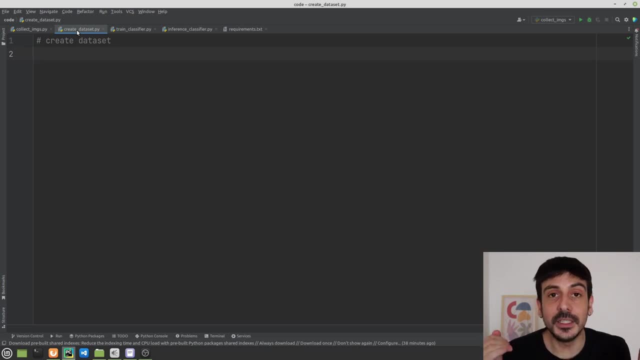 project, about the process in which we are going to be working today. This will be a three steps process And this is actually a very classical machine learning process. We are going to start with the data preparation, the data creation, Then we are going to train the model And then 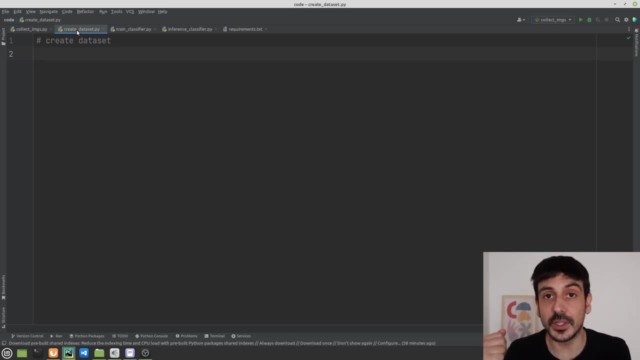 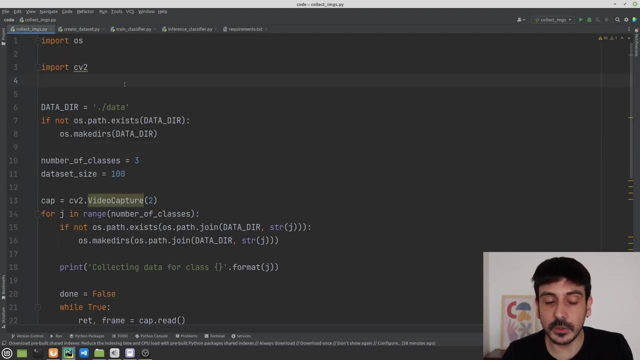 we are going to test how this model performs. So these are the three steps in which we are going to be working today. Now, in order to get started with this tutorial, I have already created a script which is going to be super, super helpful in order to create our data set. This is a script. 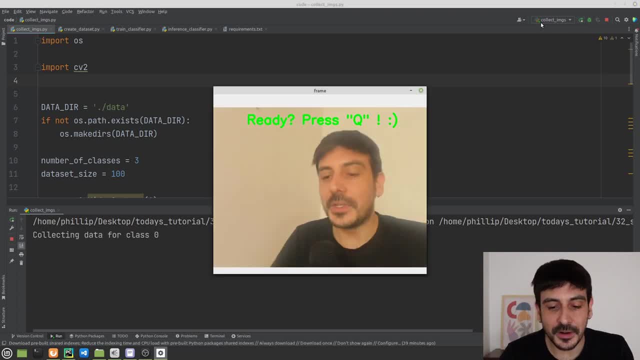 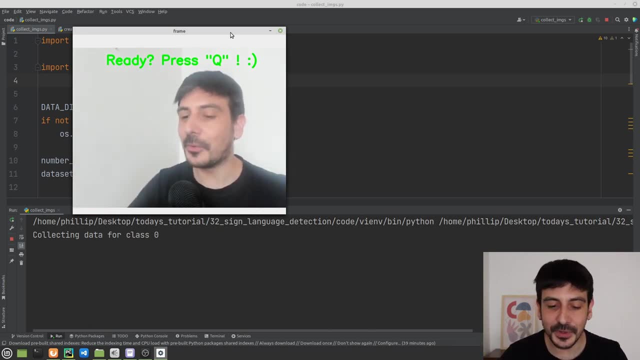 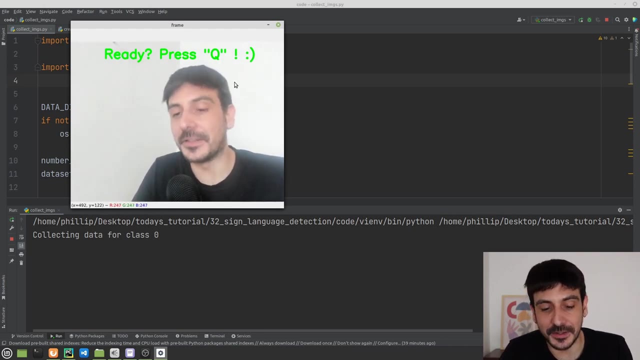 I have already created So we can save some time while we are working on today's tutorial, So we can focus our energy on everything else, because everything else will be much, much more important. So you can see that this is my webcam. As such, I have my webcam saying ready and if ready, press the letter Q. So the way we are going, 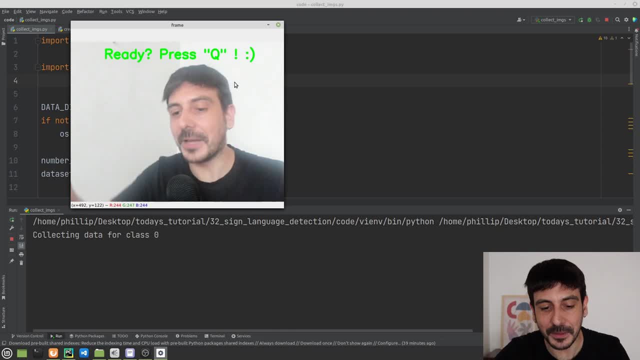 to use this script. the way we are going to use this webcam is that we are going to collect many different samples of the three symbols I shall show you Right. So what I'm going to do is, for example, for the letter A, for this symbol will represent the letter A. I'm going to do many times. 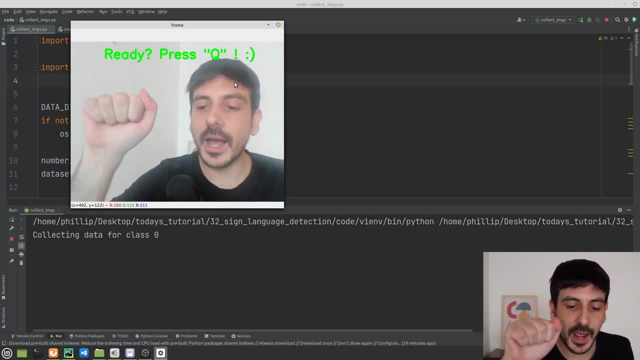 I'm going to do this process. I'm going to move my hand towards the camera and away from the camera And this way, what I'm going to do is to create many different samples, many different examples of how the letter A looks like Right? Remember, we are building a classifier and the way classifiers. 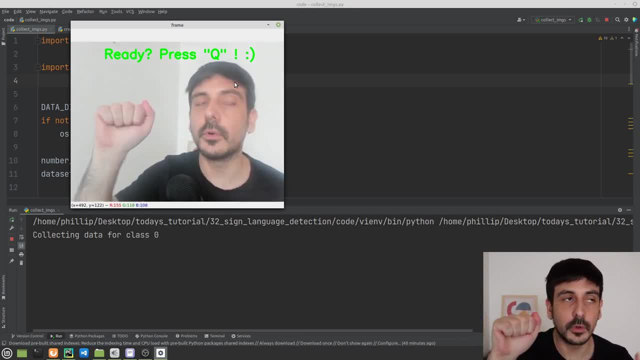 work, classifiers need data, And the more data we have, or the more diverse data we have, is going to be much better. So I am going to do this process for the letter A, Then I'm going to repeat the same process for the letter B, And then I'm going to do exactly the same process for the letter L. 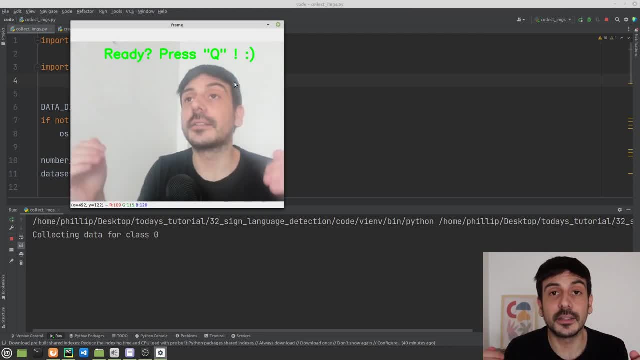 I'm going to do the same process for these three symbols And this way we are going to collect our data, We are going to generate our data set, The data set we are going to create in order to work on today's tutorial. So the idea is that, once I'm ready, I press the letter Q and I start collecting. 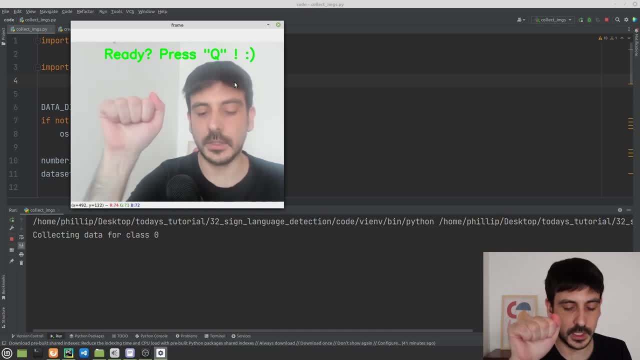 symbols. I start collecting frames for all these different symbols. So let's start there. I'm going to press the letter Q and I'm going to move my hand towards the camera and away from the camera, And that's it. So now I'm going to. 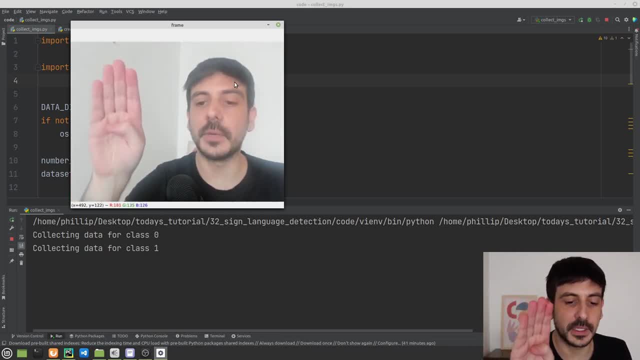 move to the next symbol, which is something like this: And I'm going to move my hand towards the camera and away from the camera And I'm going to do that for a few seconds, and that's pretty much all. I'm going to do the same with the letter L and I'm going to move my hand towards the camera. 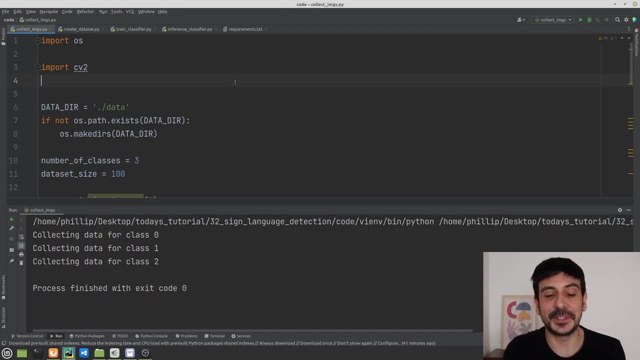 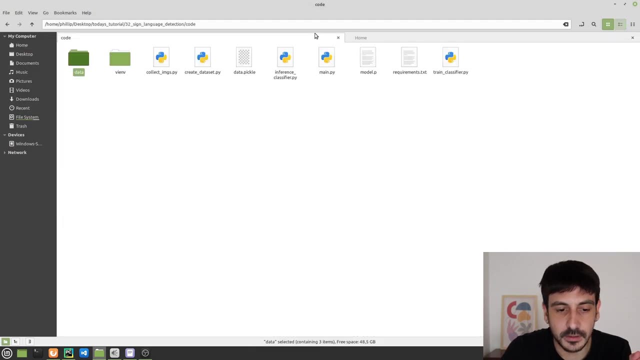 and away from the camera, And I'm going to show you in a few seconds how this data looks like. So this is pretty much all. Now let's go to this project directory and I'm going to open data And you can see I have three directories. 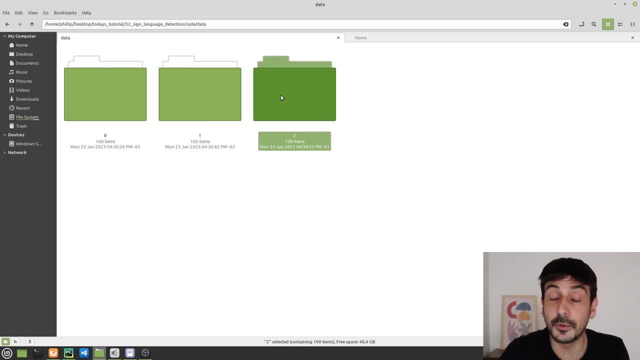 The directory called 0, another one called 1, another one called 2, And these are the three classes we are going to generate, We're going to classify today. each one of these classes is encoded into a number, into each one of these numbers and, if I open, 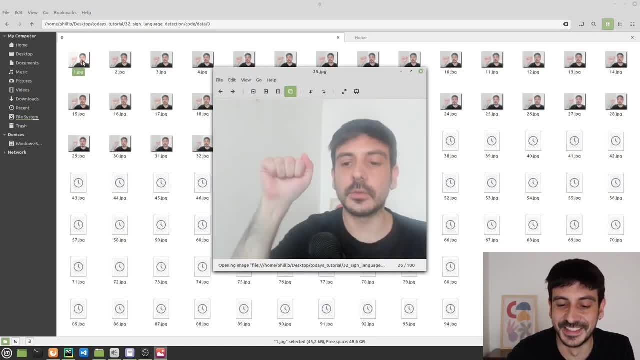 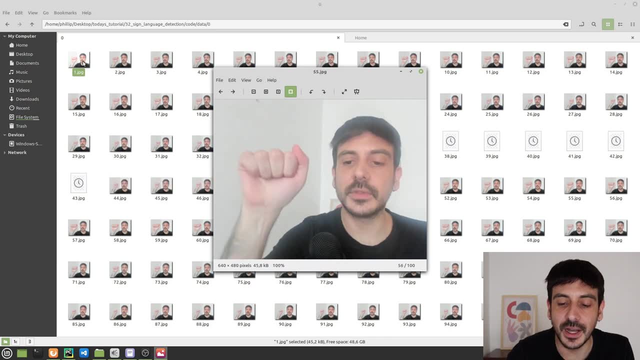 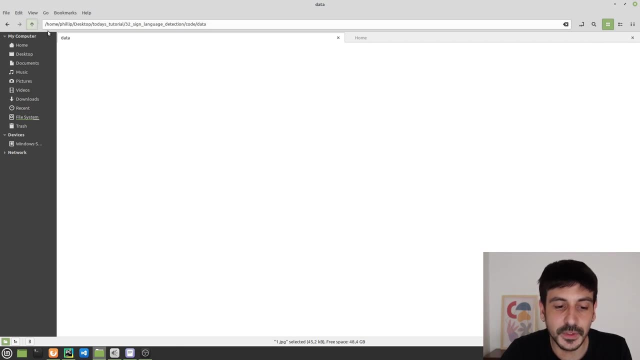 One of these directories, you can see that this is me Just doing the exact process I just did, just moving my camera towards the camera and away from the camera And while I was talking to you in this video. so these are the samples, These are the images I have just generated and for each one of these directories I have 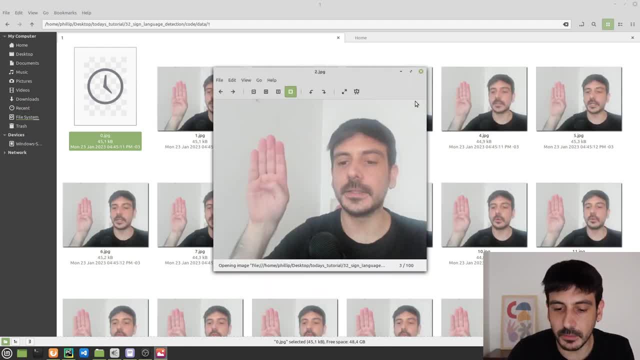 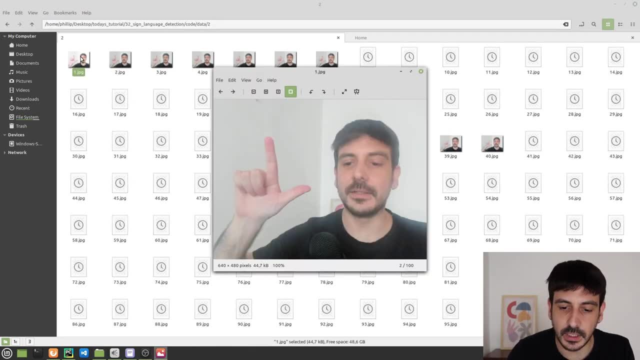 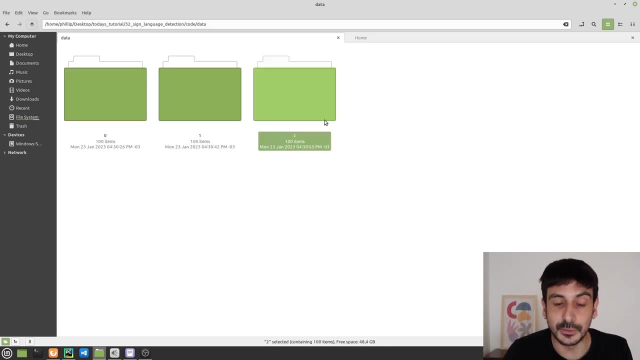 100 images, right? so I have collected 100 samples from each Category, from each class. I'm going to show you for the last class, which is exactly the same idea, But for the letter L. so this is exactly a data We are going to use in order to train our classifier. 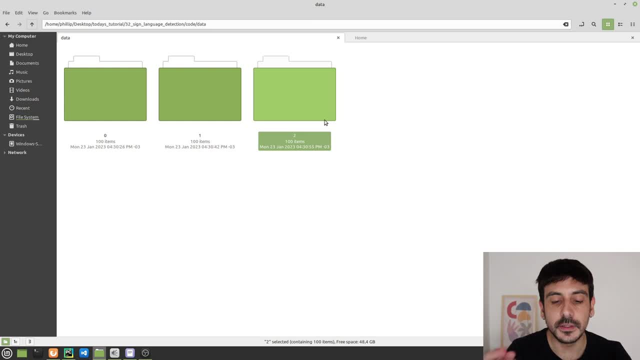 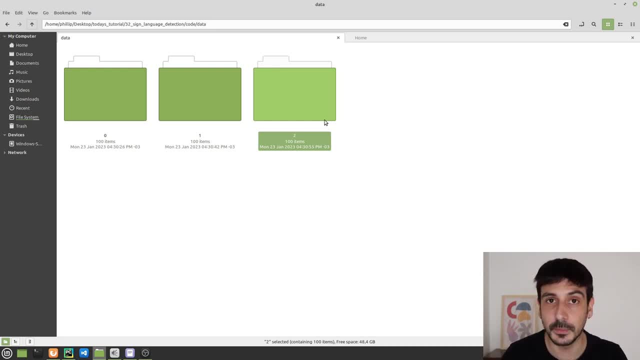 There will be many different approaches you could take in order to solve the problem. That will be always the case, given a problem. There will be many, many, many, many, many possible solutions, And the idea is that, when you are just starting on a project, the idea is that you consider some of these solutions. you just 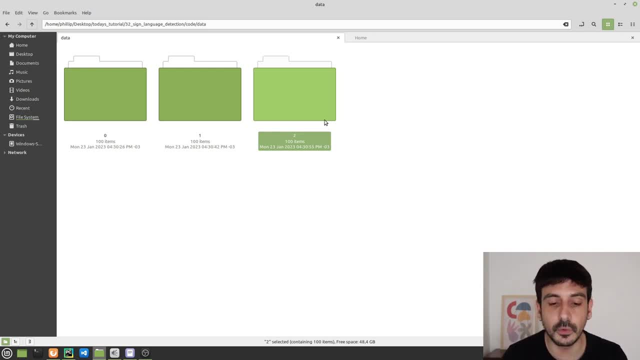 Consider all the different ways, or some of the possible ways, to solve the problem, And then you decide for the most promising approach, for the most promising way, right. For example, in this case, one of the ways we could solve this problem is by building an image classifier. 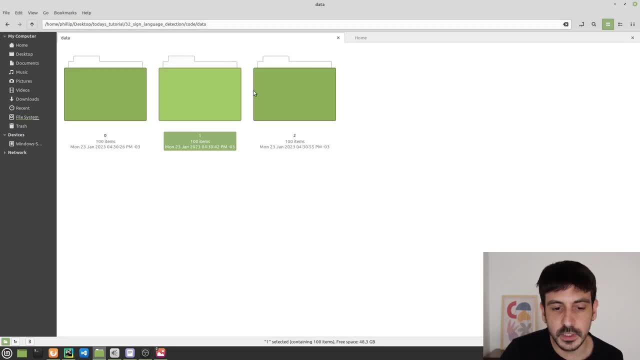 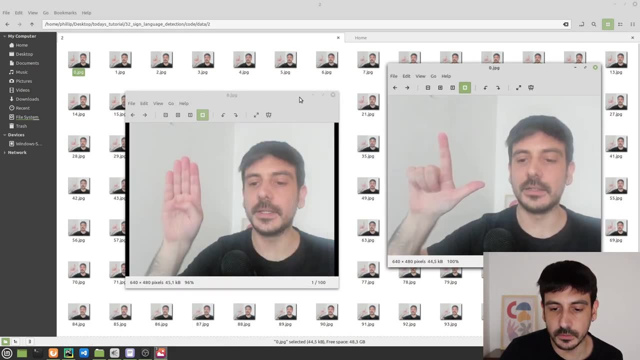 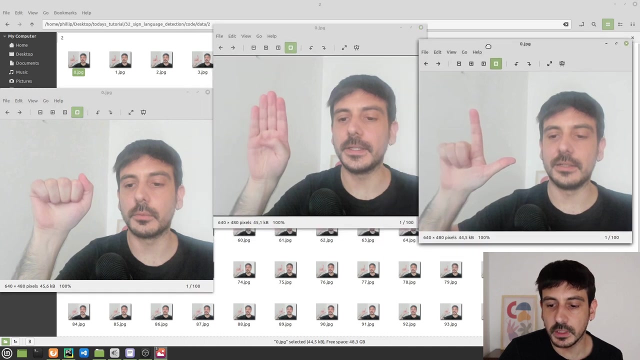 So if I open one of the frames for each category, You're going to see that Let me do something like this, one next to the other, So I can show you exactly what I mean. One of the ways we could solve this problem is by building an image classifier that takes the entire. 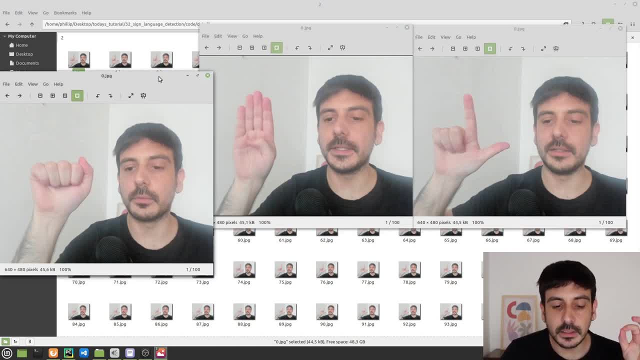 image, the entire frame, as input, and This image classifier to classify each one of these frames into different categories. So, for example, this image, the entire image, would be the letter A, Then this other image will be the letter B, And then this other image will be the letter L, and so on. right, we could label the entire frame. 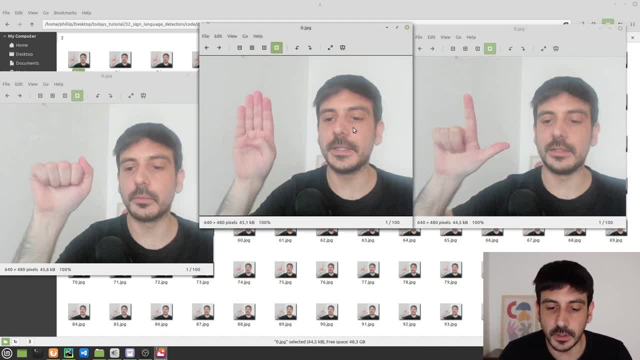 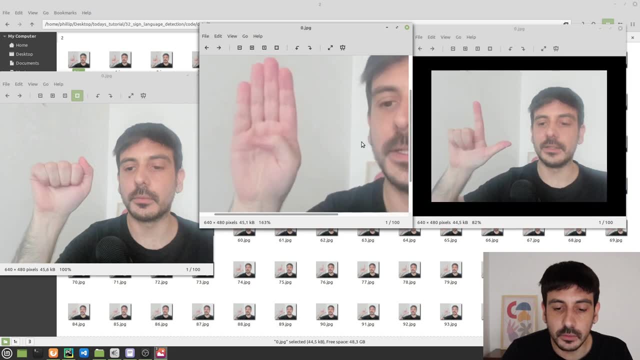 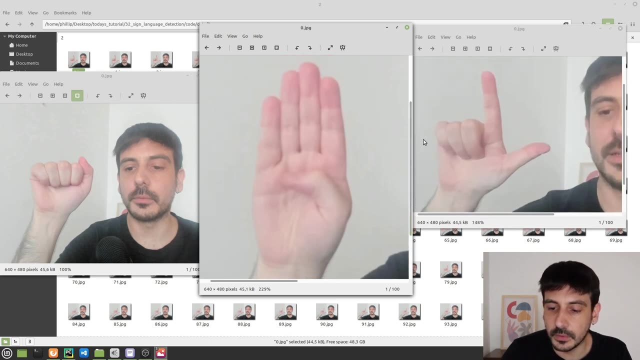 With the category, with the symbol we want to classify. that would be a way to do it, That would be an approach. then another approach would be to crop the image and to consider only The symbol we want to detect, right? so, for example, in this case we will make this crop. in this other case, 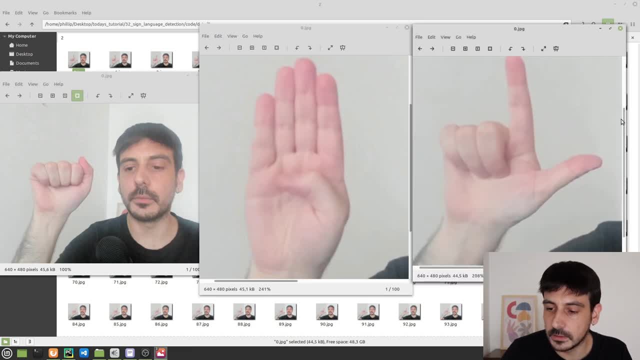 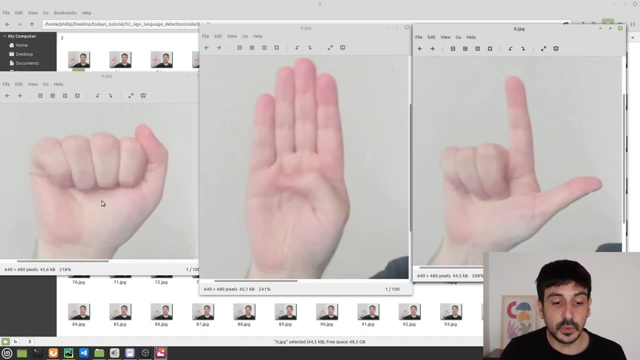 We will make this our crop, or something like it, Or something like this, and then this our case. we will make this our crop, right. so in each case, We will be Using the same approach in terms of using an image classifier, but we will be classifying. 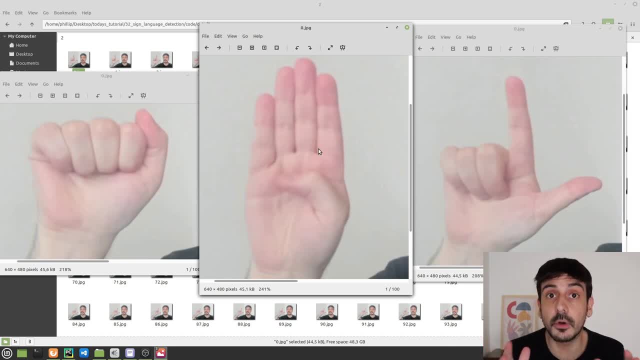 Different things right, or we will be classifying only a crop from the entire frame. So this will be another way to solve the problem and I think it makes sense. it will be a very good way to solve The problem. I'm sure we will achieve a very, very high accuracy and I'm sure we will achieve a perfect. 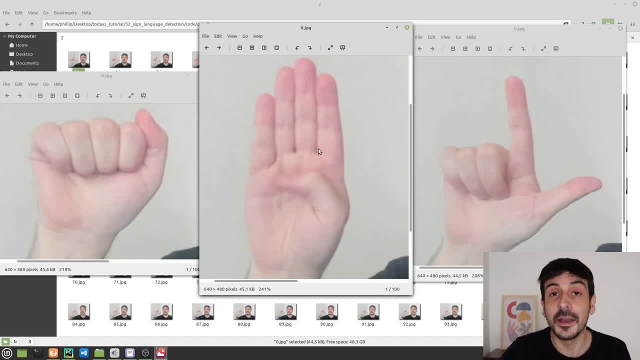 Performance, because it looks like a very good way to solve this problem. but another approach is to, Instead of using the entire image or instead of using an image, We could extract the information. we care about this image, Which is only the position of the hand right, because, if you realize, for each one of these gestures or for each one of these symbols, 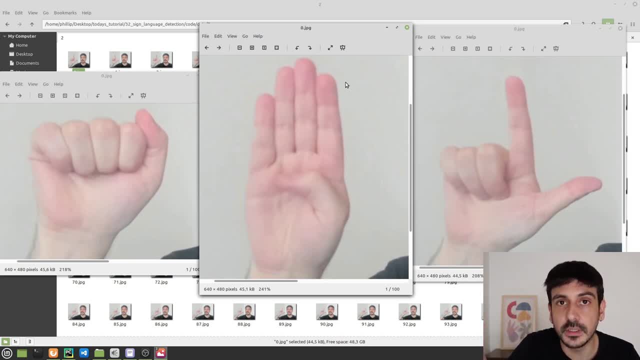 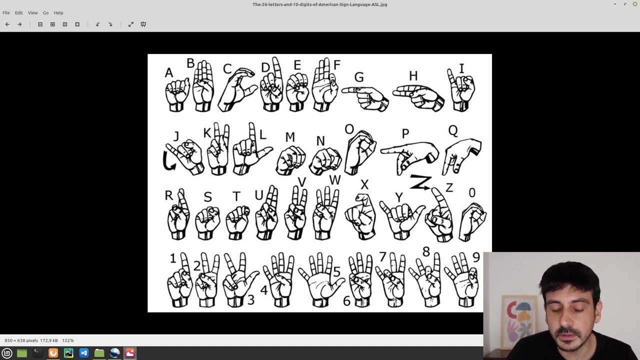 all the information is in the Position, in the posture, of all the different fingers and my hand and and so on, right. if you think about all the different symbols I show you when we started this tutorial, you will notice that all of these symbols the only difference between them, or actually the 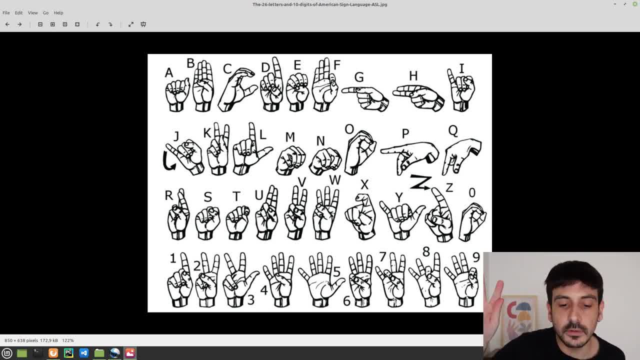 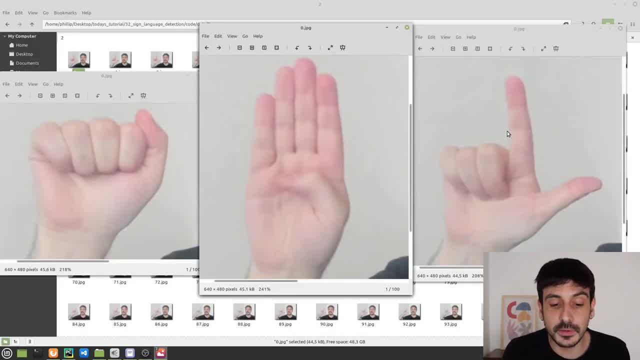 information in each one of these symbols is how the hand is located and how the Fingers are located, and if you think about your fingers or if you think about a person's Fingers, there there are not many situations or the movement we can do with our fingers. 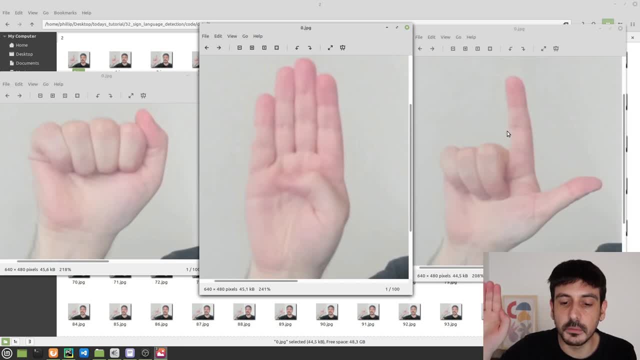 It's very constrained because we only have some possible movements right. So basically, all the information in our hands it's in the landmarks. So if we use a landmark detector, we will be extracting all the information. we care about these pictures, these images, and we will be. 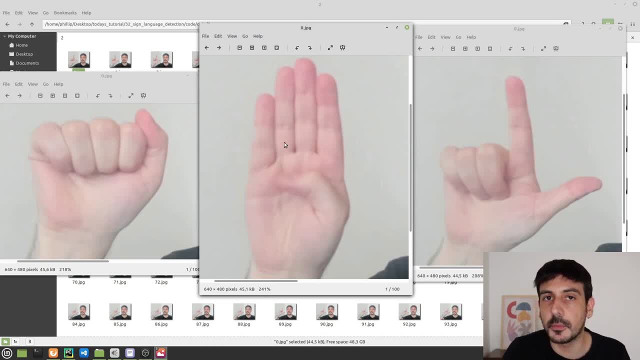 Converting, transforming each one of these images into a collection Of points, into something like 20 points or something that I don't remember exactly how many landmarks are Defined in the hand for the models we are going to use today, but it's something around 20 points. 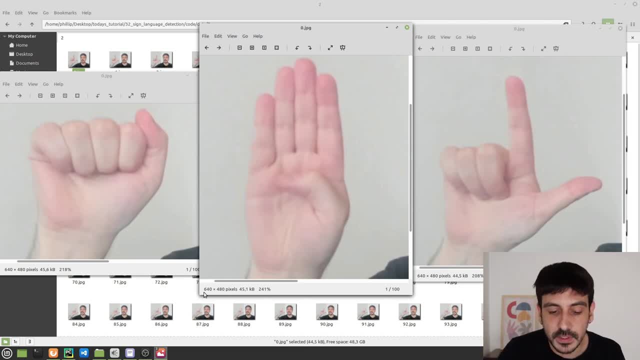 so we will be taking an entire image of 640 times 480 pixels and we will be reducing all that image, which is actually a VGR image. So it's this size multiplied by 3. we will be taking this entire Image and we will be transforming it into an array of something like 20 points or 30 points or something like that. 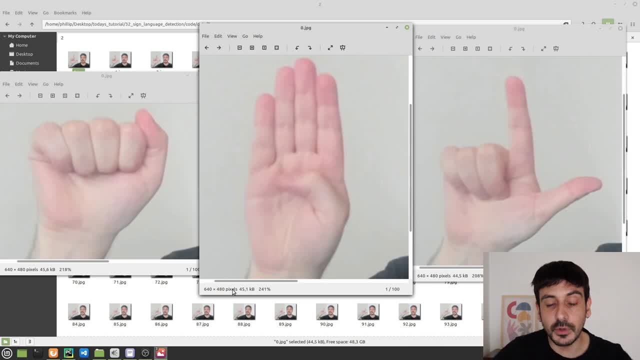 so that's a very good transformation because we are reducing the Space, the input space, the, the data we are going to classify. We are applying a dimensionality reduction technique, because we are reducing the dimensionality of our data while keeping the same information. That's very important. So that will be another approach, that will be another way to solve. 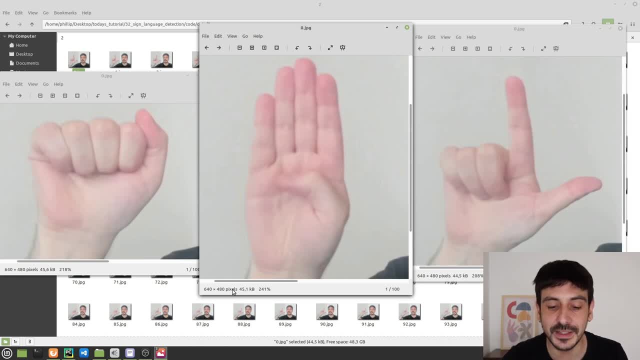 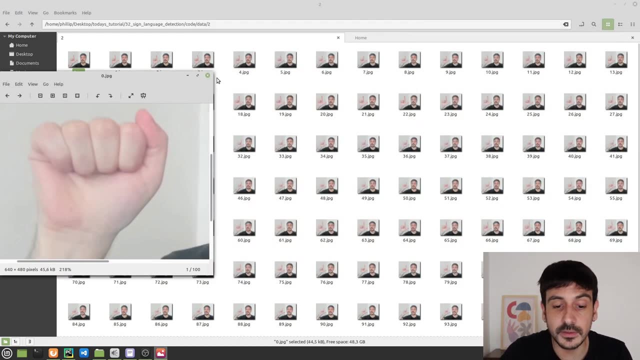 This problem and that's actually the way we are going to solve it. That's basically the classifier We are going to be building today. So that's basically something I think it's very important. I think it's one of the ways I want you to, one of the things I want you to take from this video. 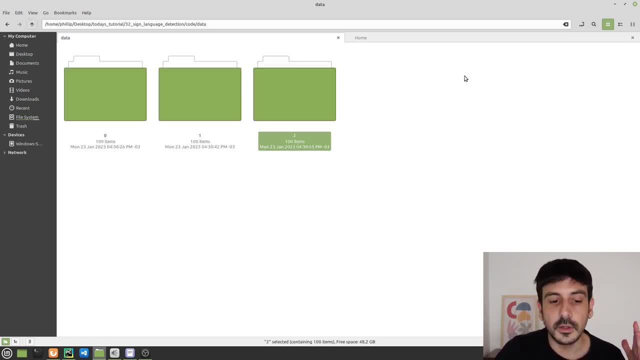 Is that, given a problem, given a project, There are many, many, many, many different ways to solve it, and it's very interesting and it's a very good exercise to consider All the different ways, or some of the different ways, to solve it and to choose the most promising one. 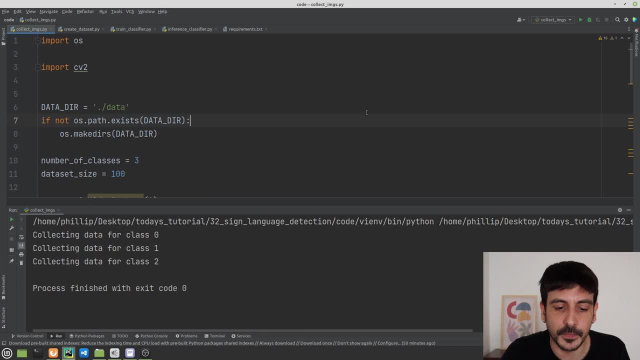 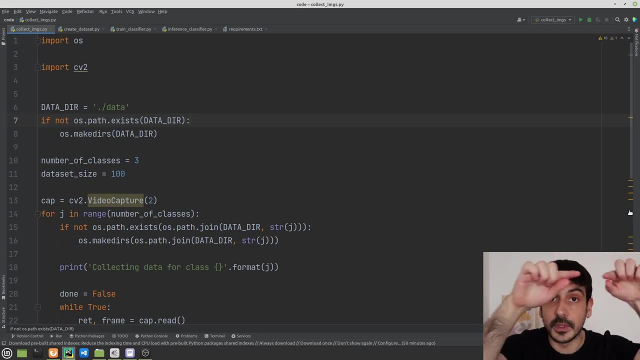 That's one of the things I want you to take from today's tutorial. in this case, We will. we could classify the entire image, We could classify only a crop of the entire image, or we could take the landmarks of the hand in each one of these images and we just classify the landmarks and that's. 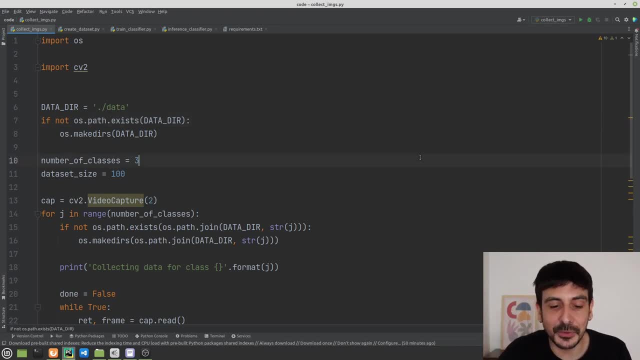 From my perspective, It's a much better approach, because the classifier is going to be much smaller and it will be much more robust as well, because The input of this classifier will be the information it needs in order to make a classification right. It will be only the position of all the different fingers and the hand and so on, and we will be removing all the unnecessary. 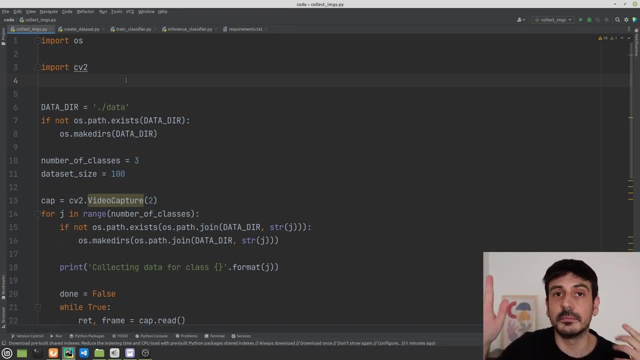 information, like all the pixels and the hand and the background and me and everything else, which is completely unnecessary In order to make the classification right. So that's the approach we are going to be taking today and this is the data in which we are going to be working into. 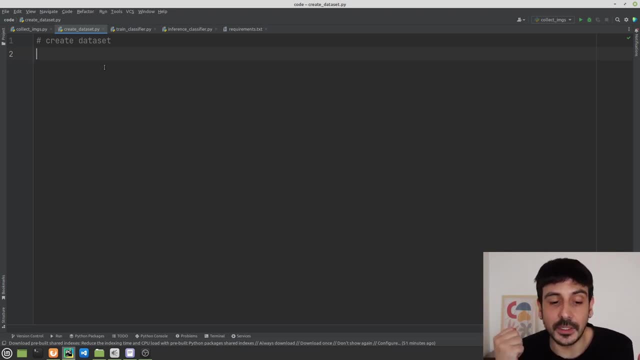 this tutorial now In order to extract the landmarks and in order to move forward with the approach I described. We are going to take all the images and we are going to do some post processing. We are going to process all these images, So we create exactly a date that we need in order to train this classifier. 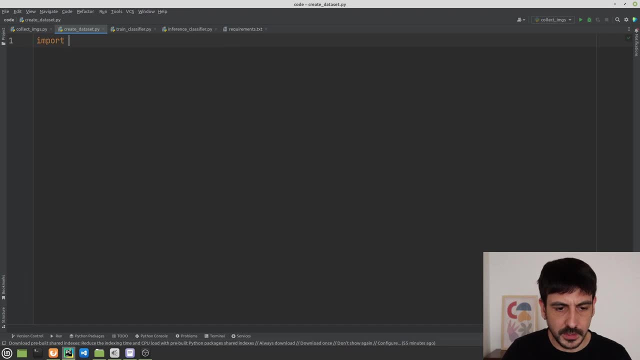 And the first thing I'm going to do is to import media pipe as MP. This is one of the libraries We are going to use. then I'm also going to import cv2 And I am going to import OS. Okay, And now what we are going to do is we are going to iterate in all the frames, in all the images I show you. 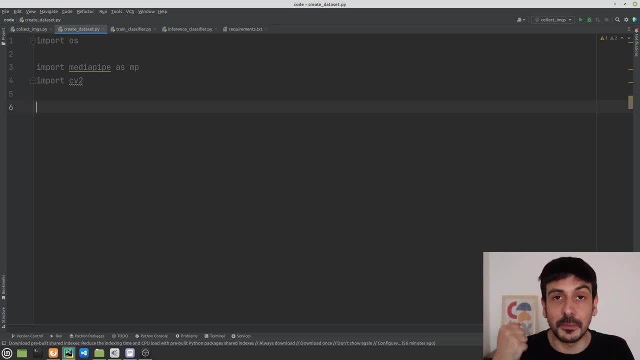 A few minutes ago, and we are going to extract the landmarks from each one of these images and we are also going to save All this data into a file We are later going to use in order to train or classifier. So let's start doing that: the data deer. I'm going to define a variable which is data deer. 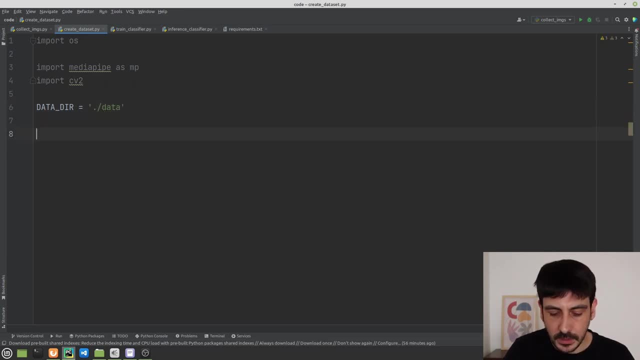 And this is located here. Okay, then, I am going to iterate in all the directories in data deer. So this will be for the ring of this deer, data deer, and I will Iterate in all the frames within this directory. So this is something like for image paths in OS, this deer and 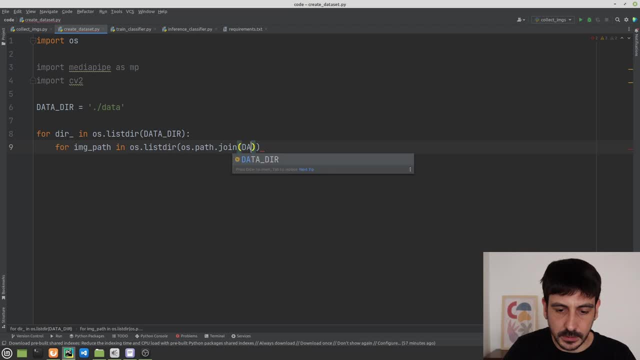 OS path. join data, deer, deer and That's basically off. Okay, and, And I am going to define this image path as dot path: join data, deer, deer and image paths And I'm going to create a variable which is image. an image will be cv2 in read and this image path. okay, now I'm going to convert the image into. 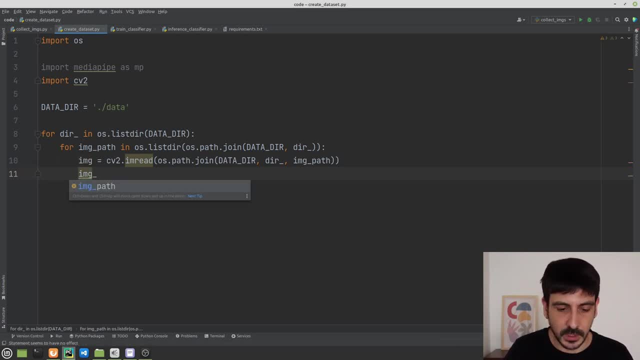 VGR or actually into RGB. it's already into VGR because we need to convert this image into RGB in order to input the image into media pipe. when we are working with with media pipe, all the landmark detection is always on RGB. so as we are reading the image in VGR, we definitely need to convert it into RGB. 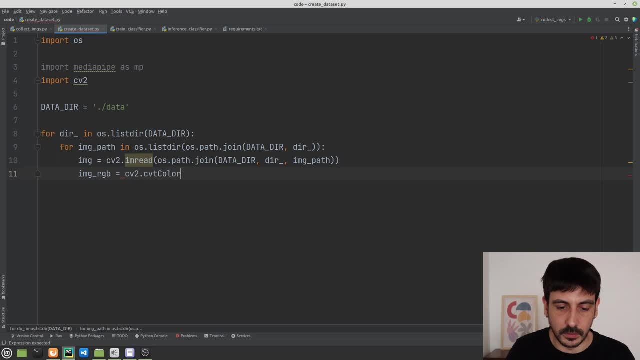 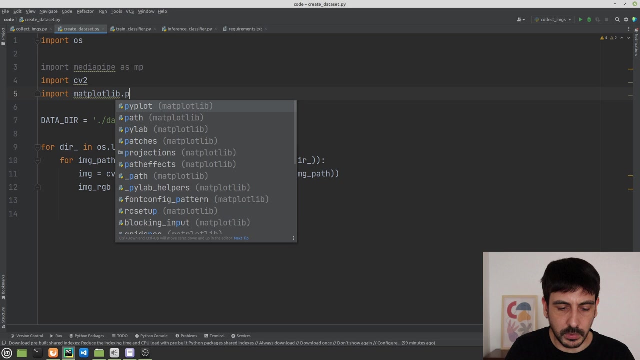 so this will be cv2- convert color image and then cv2- color VGR to RGB. okay, so this is pretty much all. so this is the images we are reading from our data directory, and now I'm going to import matplotlibpyplot because let's plot how these images look like. 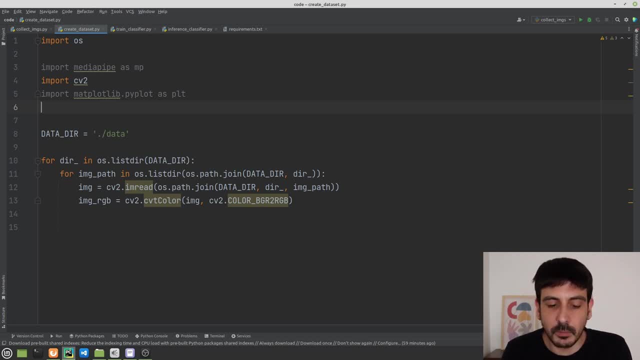 I am going to extract landmarks in a few minutes, but for now, let's just plot these images in order to make sure everything is working properly. so I'm just going to plot a few. I'm going to plot one for each directory. so I am going to do something like this, so I only take the first one. okay, and now? 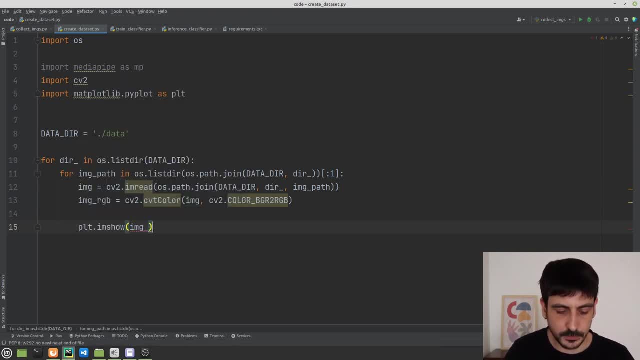 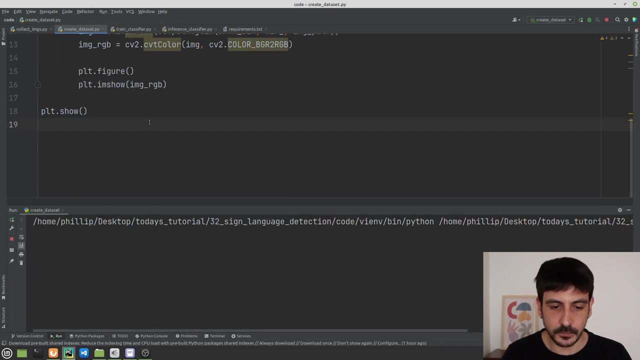 this is in show image RGB. remember that a matplotlib also requires the image into RGB in order to plot this image using matplotlib. this will be plotfigure and then plotshow and let's see what happens. let's see if everything is working properly. okay, perfect, so we are. 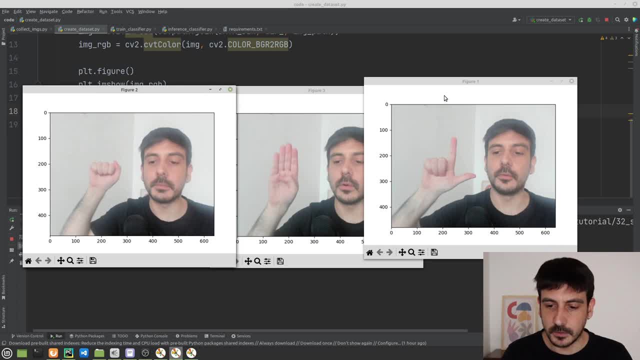 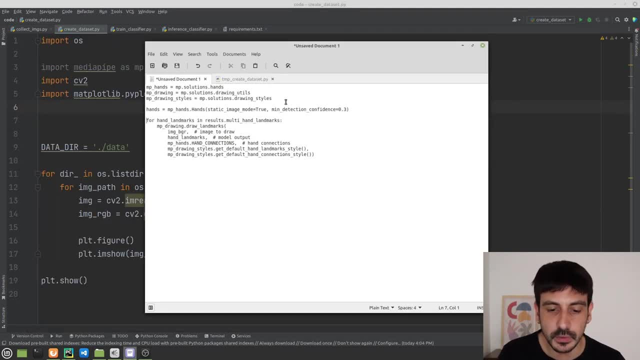 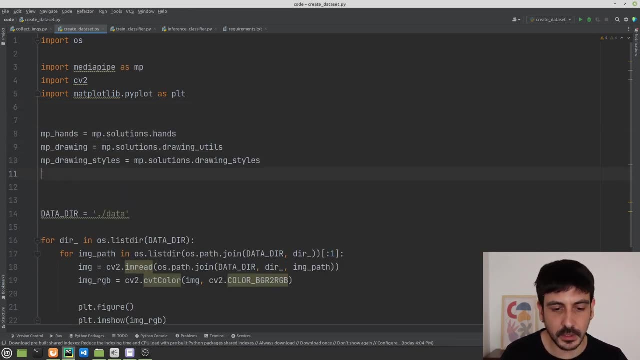 plotting a frame from each class, from the three directories, and everything seems to be working properly so far. now let me show you three options we are going to use, which are these three sentences I have over here. I'm just going to copy and paste everything. everything is already ready in this. 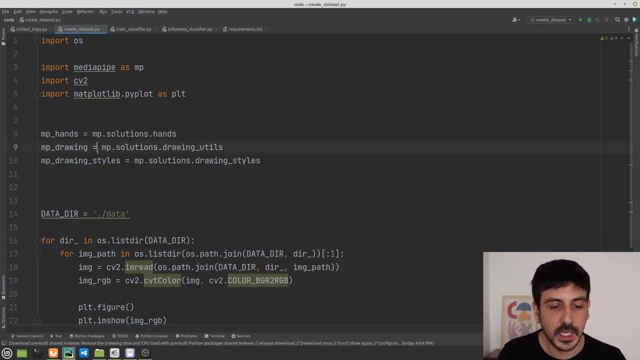 notepad, so we don't really lose time defining these objects. and this is basically three, three objects which are going to be super, super useful in order to detect all the landmarks and in order to draw these landmarks on top of the images. we don't really need to draw the landmarks on top of the images in order. 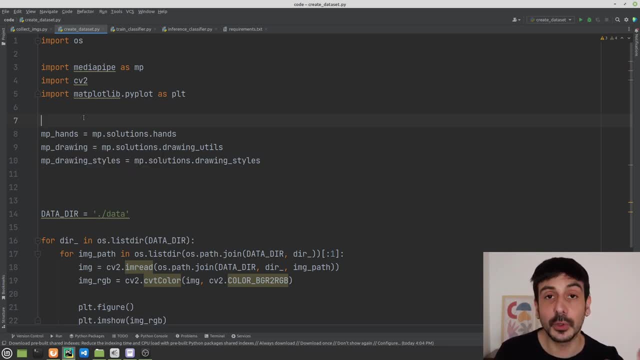 to do our classification, but I'm going to do it only to show you how this landmarks look like. so these are the three objects we are going to use, and now let's define an object, the hands detector, which is something like this: this will be, if I'm not mistaken, a phandshands, and then the variables. 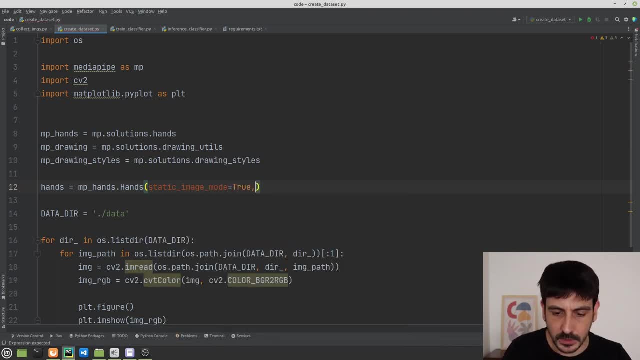 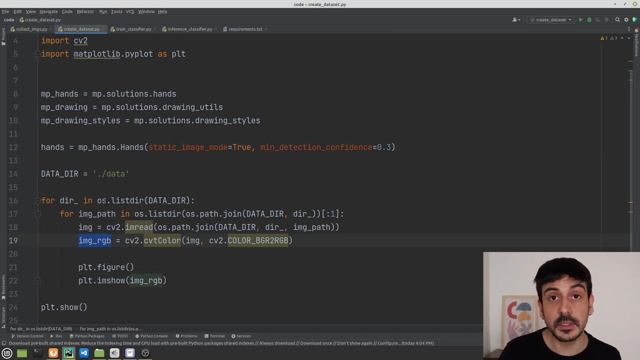 or something like static image mode. true, and then confidence mean detection confidence, which is: we're going to use 0.3. okay, so this is the model we are going to use. and now going back here, remember, this is the image. this is the image we have. 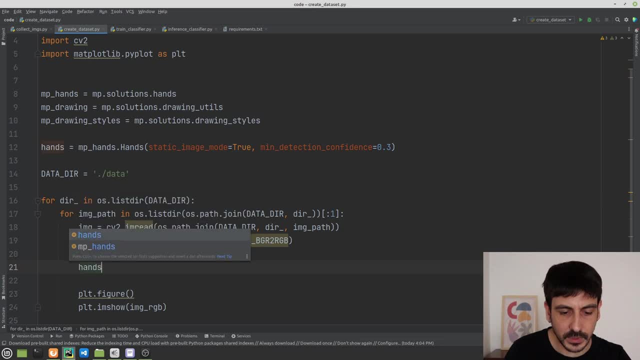 converted into RGB. and now we are going to do something. it is we're going to say hands, dot process, and we are going to take this image here, and what we are doing here is to detect all the landmarks into this image. right, that's exactly what we are doing with this sentence, and now the only thing we need 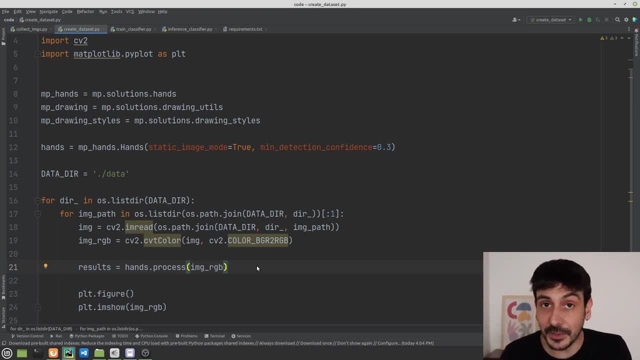 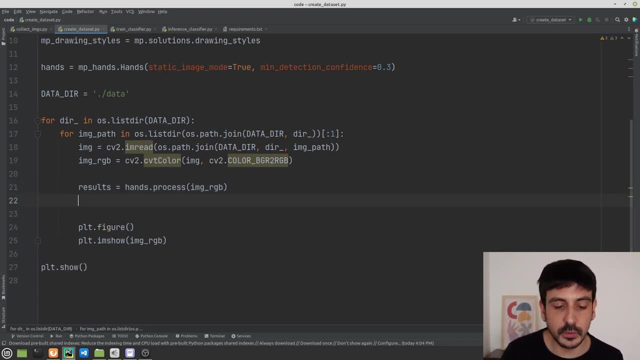 to do is to iterate in the landmarks, in all the landmarks we have detected in this image, and for that, maybe the best way to do it, in order to move one step at a time, is to show you how these landmarks look like. so let me get back. 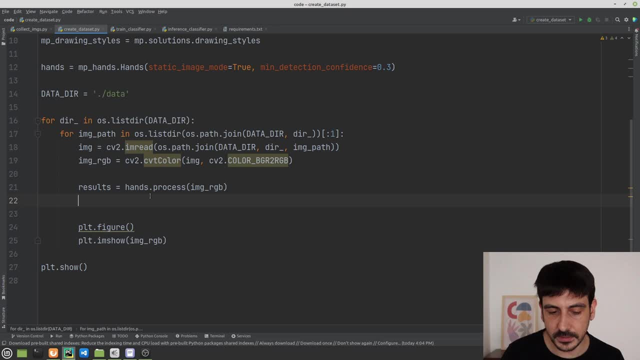 here and I am just going to copy and paste this function, which is going to be a much. it's a much better way to do it. I'm just going to copy and paste it so we don't really lose time to use it. so I hope this video will be useful for you. Thank you. 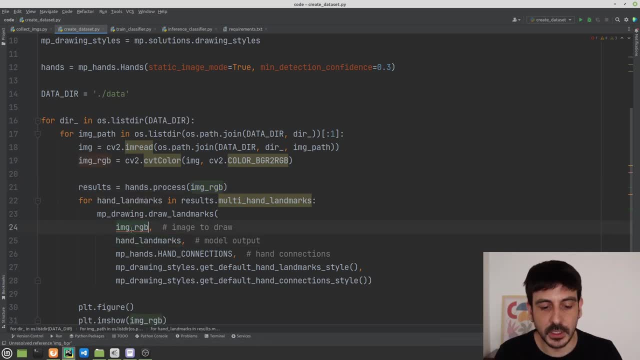 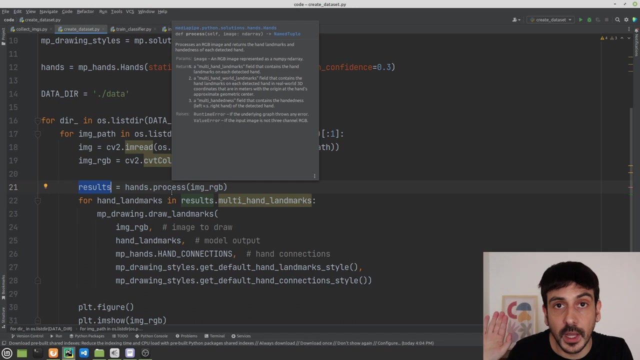 to coding this function from scratch. So basically, you can see that this is iterating in all the results we have from this hand detection we are doing here because, remember, we will be detecting only one hand or two hands or no hands at all. So it makes perfect sense to iterate. 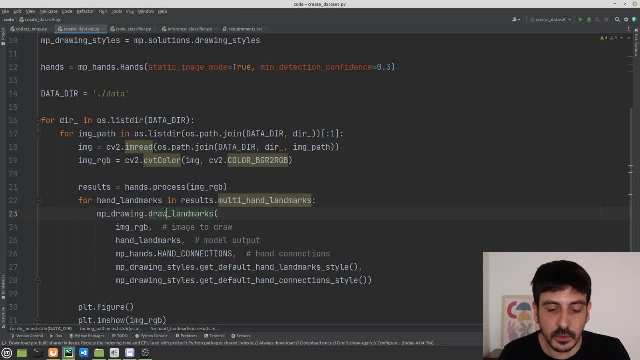 in all the different results And then, for each one of our results, we are going to draw the landmarks. And this is basically the way to do it: by calling this function with these arguments. Remember, everything will be available in the repository for today's tutorial. 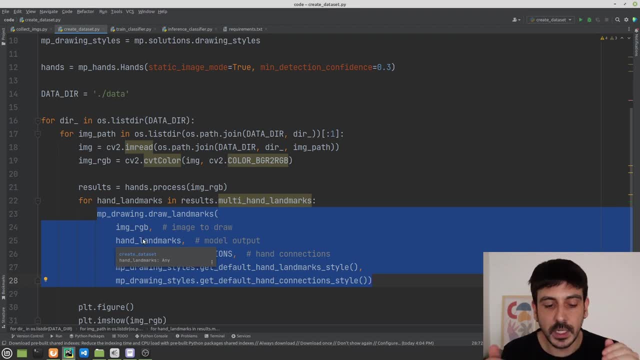 So you can just take all the code from this repository and you can just take everything from there For now, just follow along, So you just can follow the entire process, and then you can just go back to the code by looking at the repository. 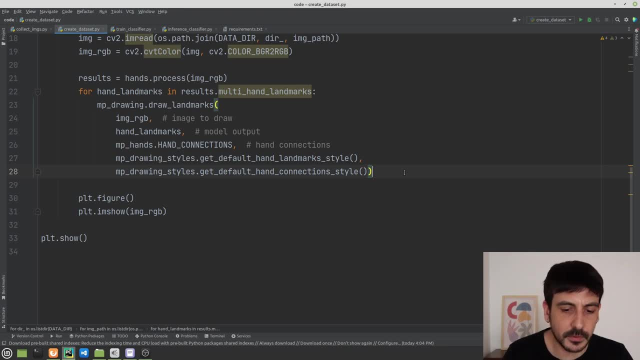 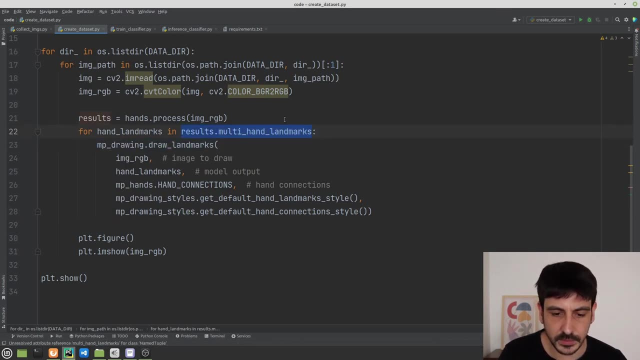 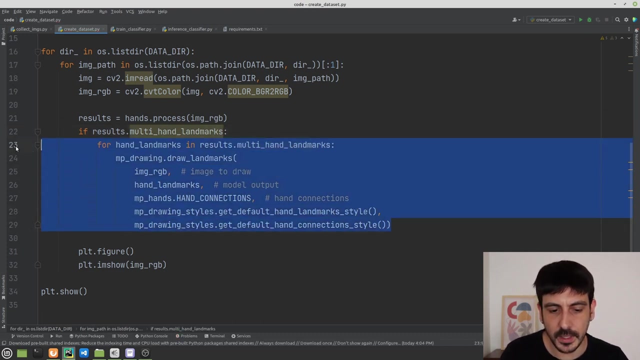 So this is the landmark drawing, and this will be pretty much all, If I'm not mistaken. let me just run this code to see what happens. I have to do something else, which is I need to ask if we have detected at least one hand right. 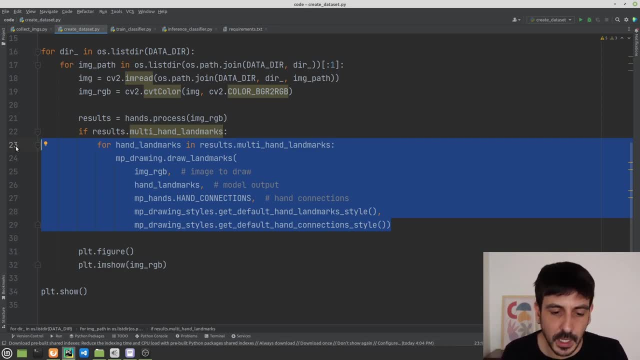 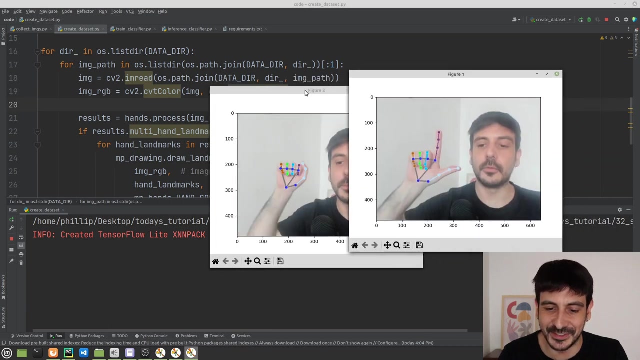 Because we could be detecting no hand at all And that could be a problem for what we are going to do later on. So let's just run this script, Let's see what happens. We are perfect, It's just perfect. You can see that we are detecting exactly. 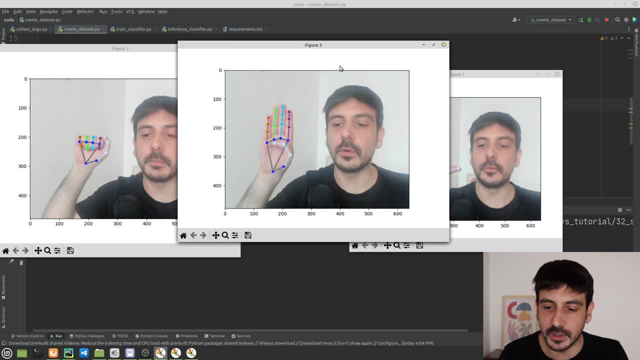 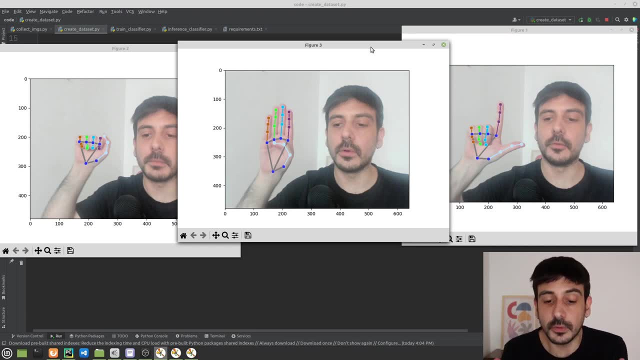 the position of the hand and we are just detecting exactly all the different landmarks. You can see that we have many different colors. The style we are using in order to draw these landmarks, it's just giving us all these different colors, So we know exactly all the different fingers and so on. 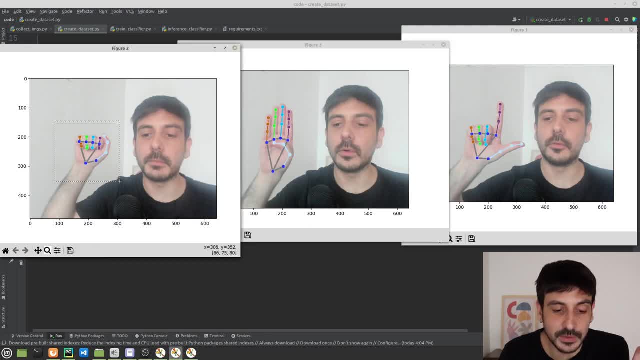 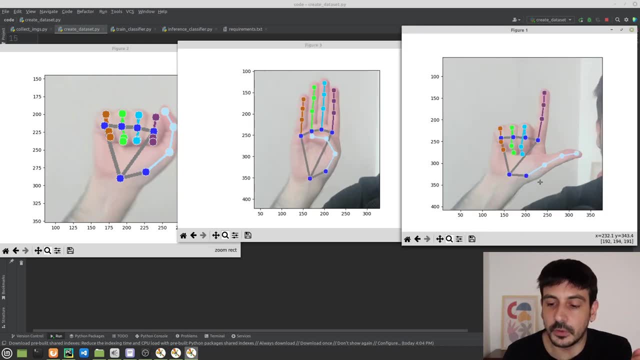 So these are exactly the landmarks we are going to use into this tutorial. We are going to take away a few accessories to take all this information and we are going to draw the we're going to build our classifier with this information. so this is only to show you how these 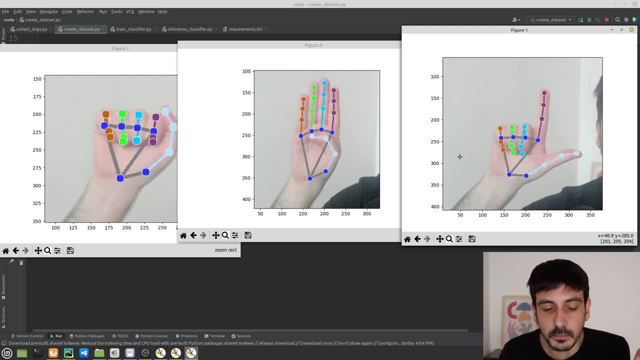 landmarks look like, and this is what I mean when I say that these landmarks contain absolutely all the information we need in order to be work on to a tutorial, in order to build this classifier, because take a look only at the landmarks, don't take a look at the image itself at my hand, but take a look. 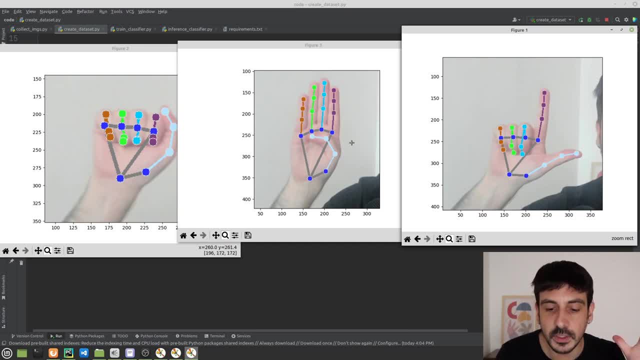 only at the landmarks and you can see that all the information we need it's in the landmarks, right. for example, in this case, for classifying the L, we will need to take a look what happens here, what happens in this section, with these four landmarks. if we have a situation like this, where this finger it's like up and 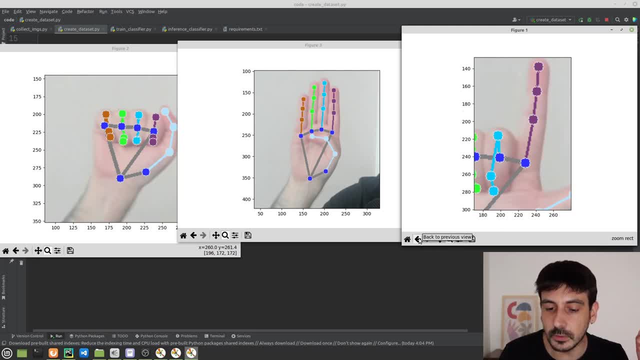 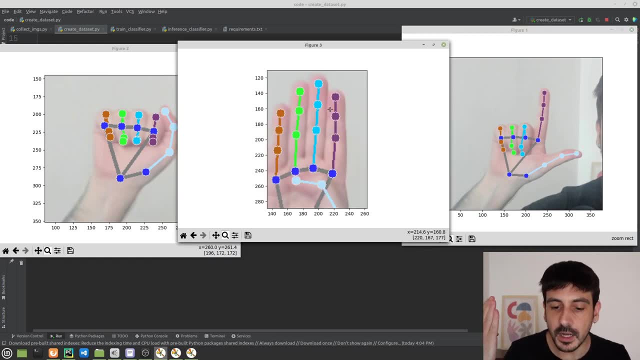 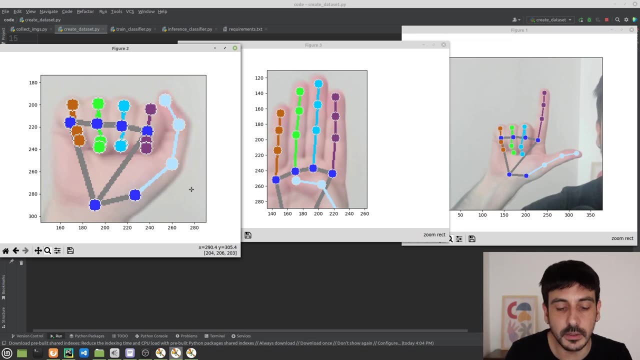 then all the other fingers are down, then that's pretty much all we need to know in order to make this classification. and then if we go here, if we notice these four fingers are up, this means we are in this situation. and if we are in this or situation with all the different fingers like this, then we 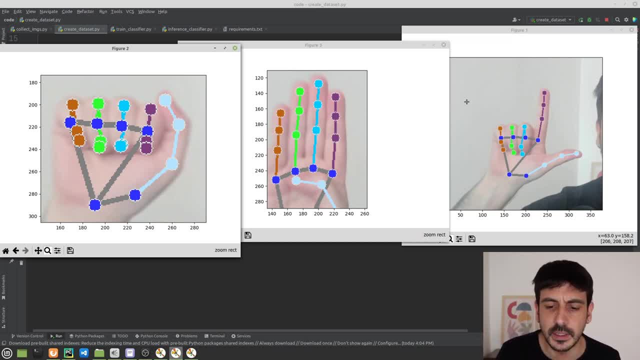 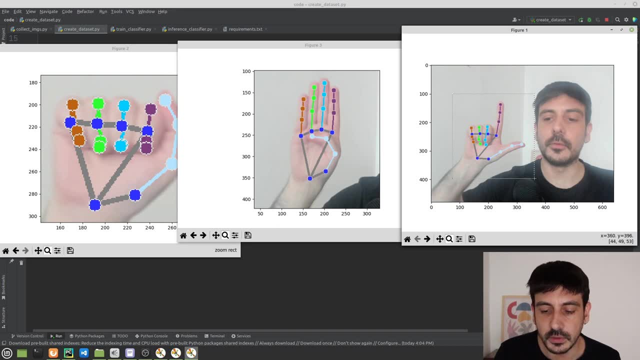 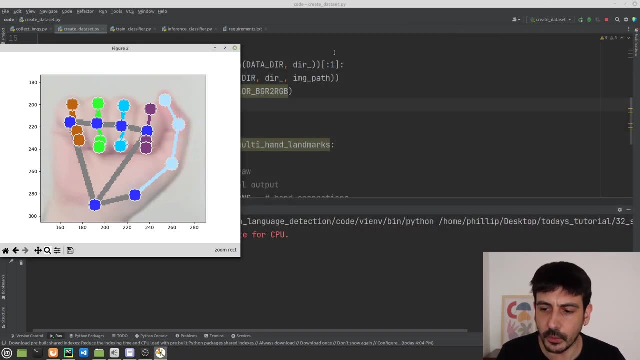 are here, but absolutely all the information we need it's in the landmarks, so it is only to show you how it looks like, and it will be exactly the same situation with absolutely any other symbol we choose. the information will be in the landmarks. and now let's continue. we don't really need to do a drawing. the 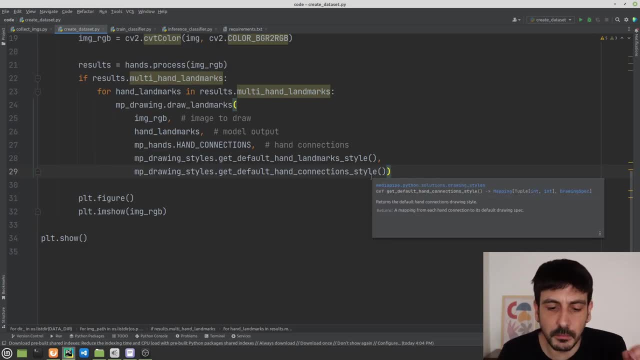 only reason I did the drawing was to show you how this looks like, but we don't really need it, so let's continue. what we were going to do now is: I am just going to remove these parts. yeah, because we don't really need it. I'm going to remove all the drawing. I'm 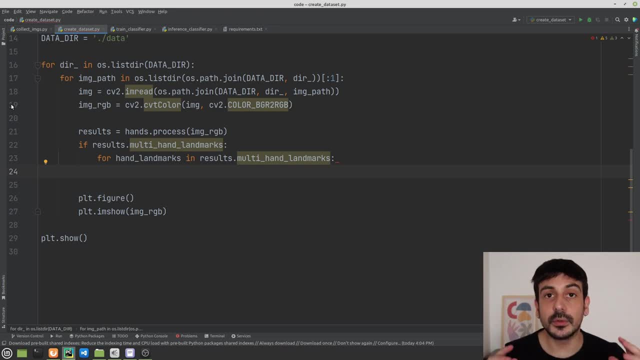 going to keep everything else and what I'm going to do is I'm going to take the entire landmarks and I'm going to create an array from all the landmarks. right, I'm going to take all the image and from each image I want to have an array with. 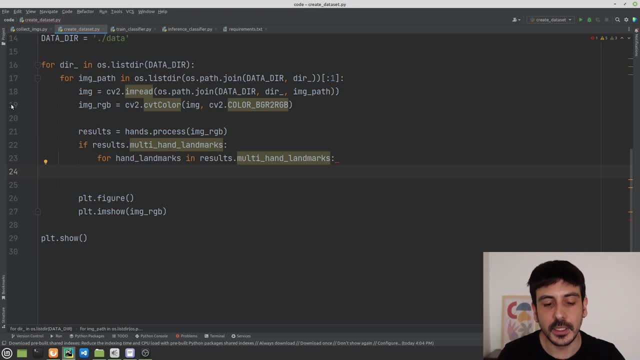 the information of the image in the whole area. so I'm going to create an array and with the information of the information of the, absolutely all the landmarks we have detected, right. so in order to go one step at a time, I'm going to iterate for e in range: the length of hand landmarks dot. 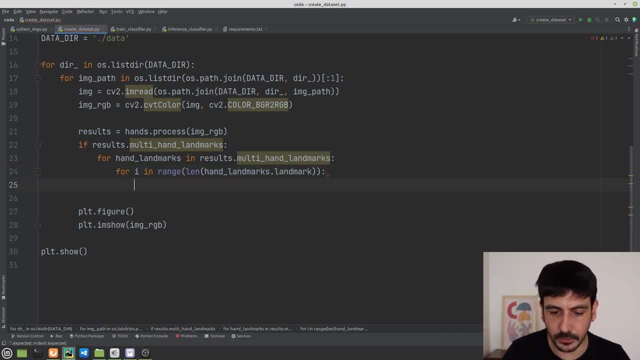 landmark and I'm going to show you how this look like. I am going to print this value and this is going to give us the value of all the landmarks. I'm going to show you how it looks like first, and then I'm going to do something with them. 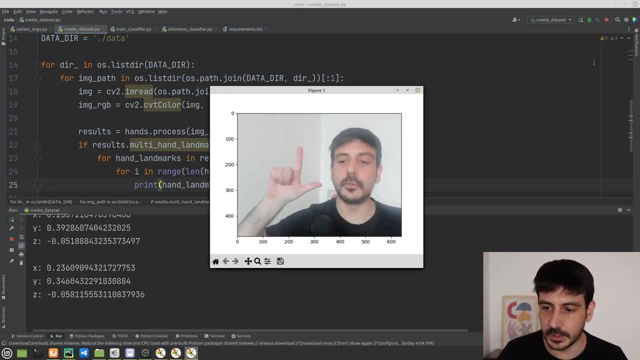 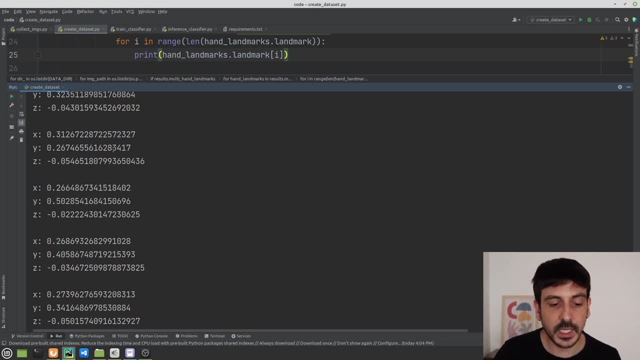 okay, we don't really need to plot the images anymore, but we have the images too, and you can see that for each one of these landmarks we have three values: X, Y and Z, and these are all the values which define exactly the position of each one of our landmarks. so we are going to use only the X and the Y coordinates, which 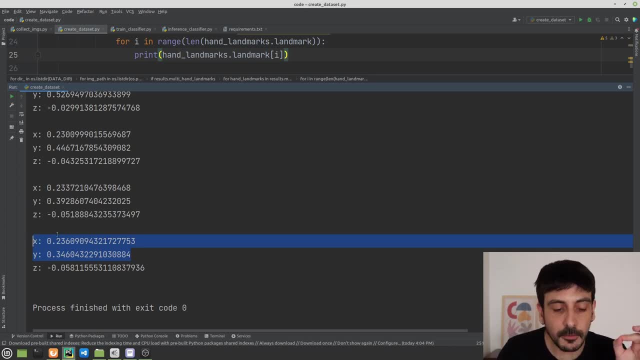 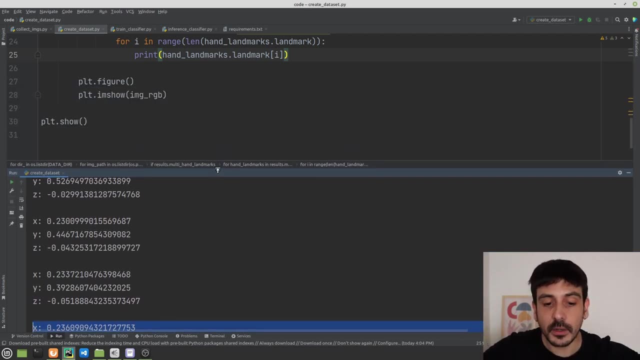 are the horizontal and the vertical coordinates, and from this information we are going to create an array, a very long array, and then we are going to train the classifier and we're going to inference this classifier by considering this array of landmarks, all on right. so we have an image, we detect the landmarks, 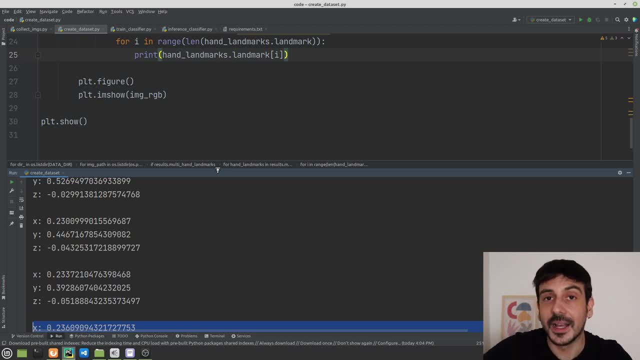 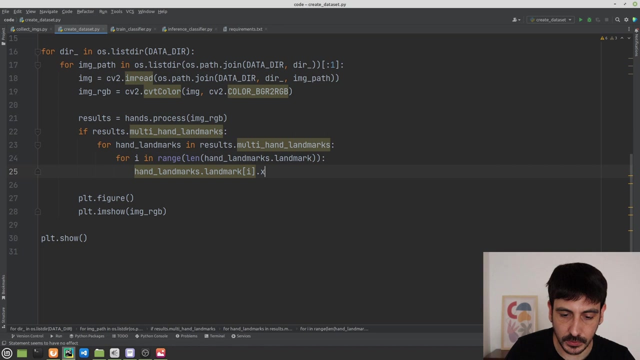 and then we take these landmarks into a very, very long array and that's the array we are going to consider in order to train our classifier right. that's the process we are taking and we are taking everything one step at a time. now we are going to look at the filtered video, so we have to say we are going to look at. 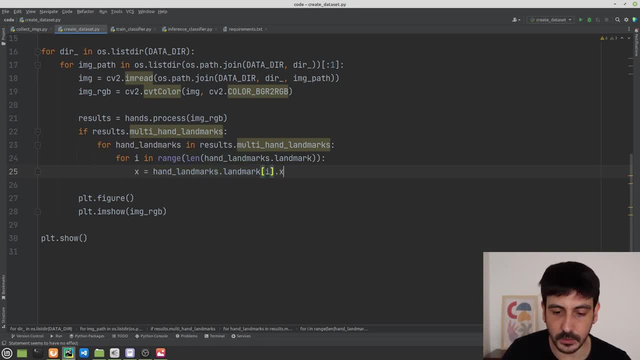 this database name, right, and we mean that we are going to allow the tables to be in this database name. we are seeing. you know that we are going to call it. I will create a new. represents figurological, אבל you don't have to apply your sajauuuu. you can go with polygons, but you can. 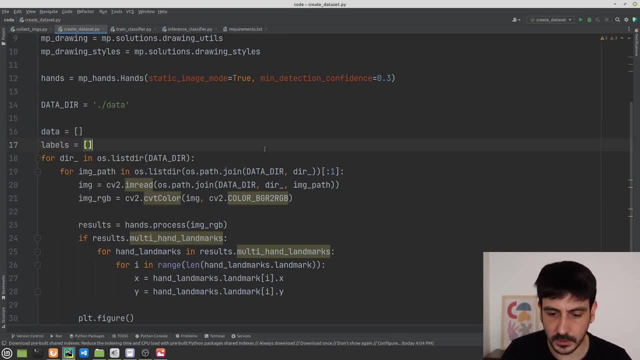 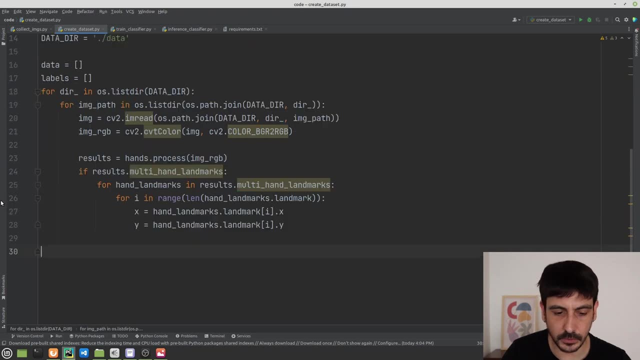 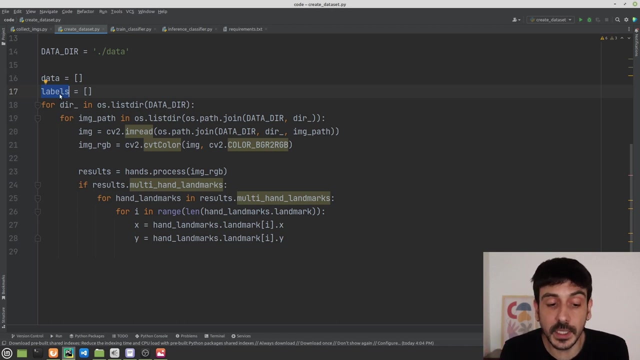 apply your drawing, bring to this where a' I am going to look for the'm한테 etwas. I Galilean that and I'm not going to plot it anymore. so we have defined these two variables, which are the variables which are going to contain all the 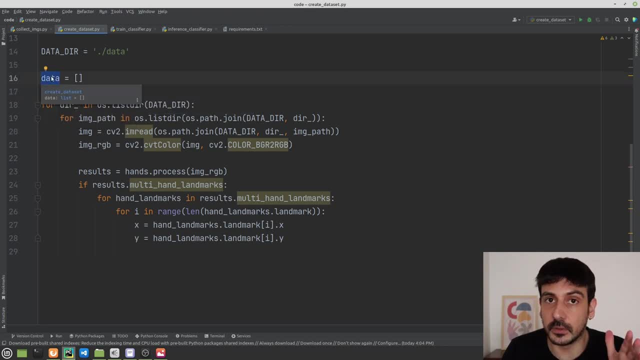 information, right, the data, which is the data we are going to produce in order to make this classification, and then the labels, which are the category for each one of these images, for each one of these data points. so, this how we are going to do it, we are iterating in all the images, for each image. I'm going to 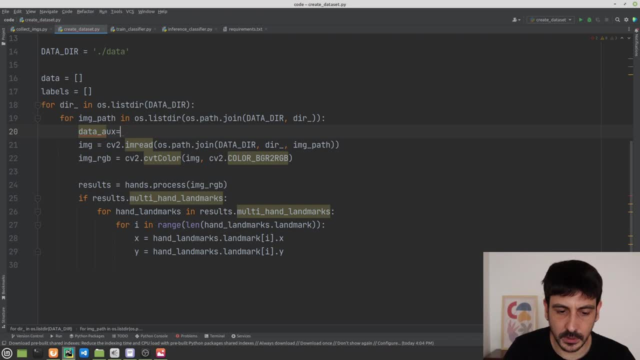 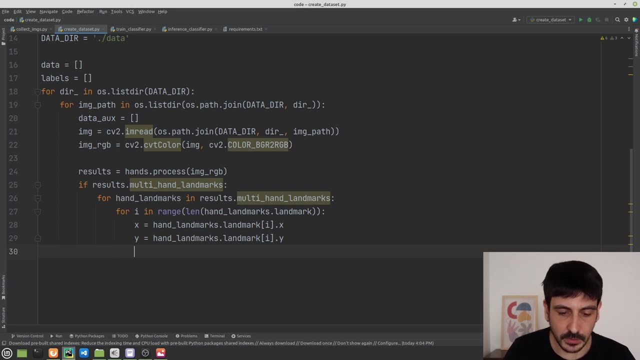 create an array which is data aux, and this is an empty array for now. and let me show you exactly what we are going to save here. this is where we are going to save the X and the Y coordinates, so something like this X, and then something like this with Y right, and then at the 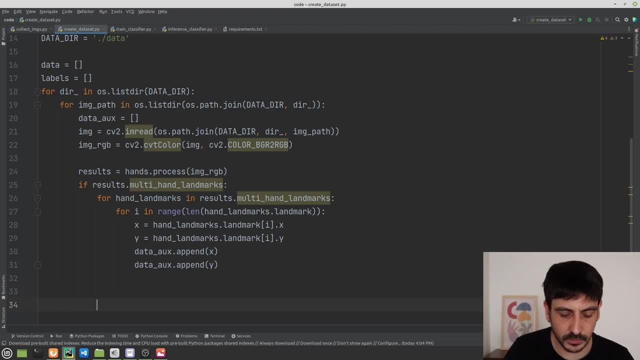 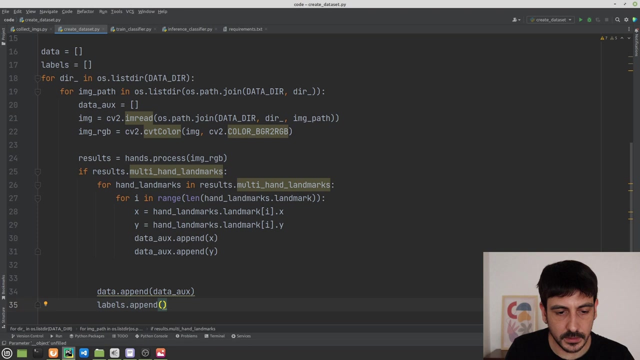 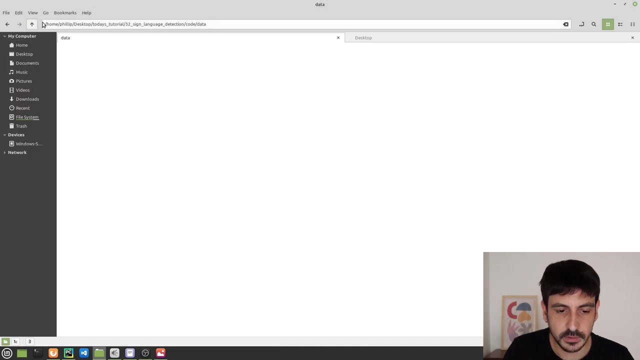 end of the entire iter. we are going to do something like data- dot append, data aux, and then labels- dot append, and then dir, which is the category right. remember that we have three categories. we have three directories. one of them is called 0, the other one is called 1 and the other one is called 2, and each one of this directories contains the another categories. one are called two and each one of these directories contains the other ones. two are being called one and each one of these I against a scale 함f meeting and, as I just explain, so if break for many. 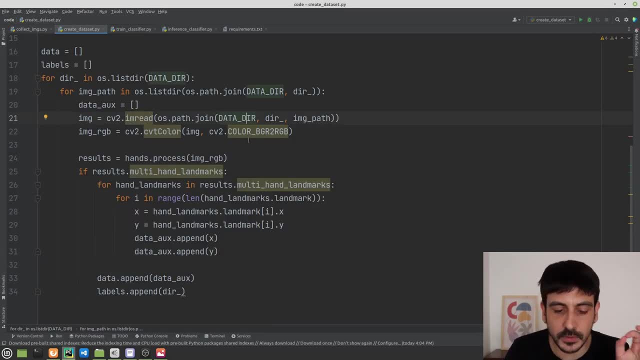 for many, each one of our symbols. so the symbol is encoded into the name of the directory. so this is exactly what we need to do for each one of our images. we are extracting all the landmarks, we are creating a very long array with all these landmarks and then this very long array is going to represent 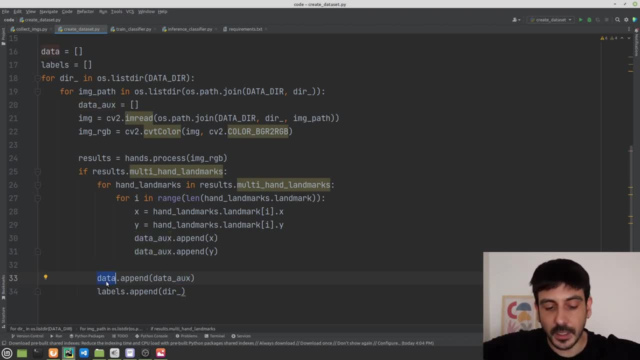 our image. right, we are going to create a, an entire list with all these different arrays, and then the labels will be the name of the directory of each one of these images. and doing so, we are creating our data set. doing so, we are creating the data set we need in order to train our classifier. 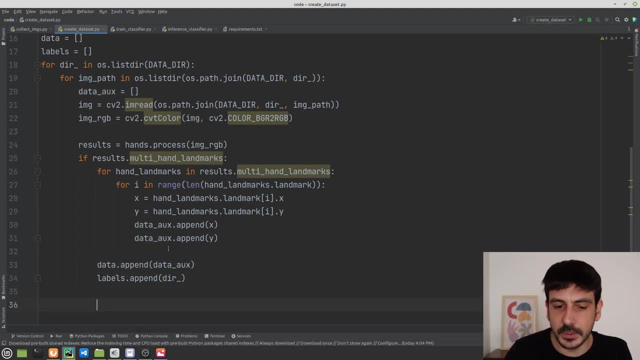 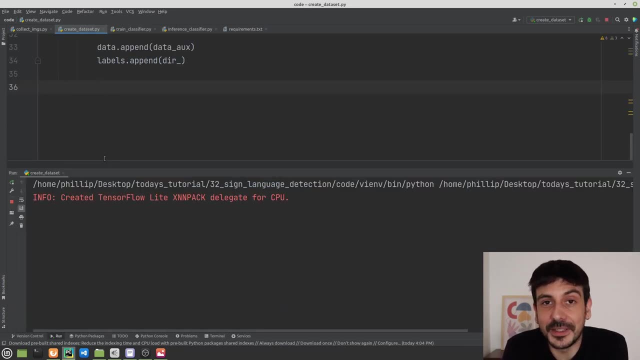 so that's pretty much all now. let's see if this works properly, because we have done many, many different things and there could be- there are many places in which we could have made a mistake, so let's see what happens. okay, everything was supported, successfully executed, so everything seems to be okay. so what i'm going to do now is i'm going to 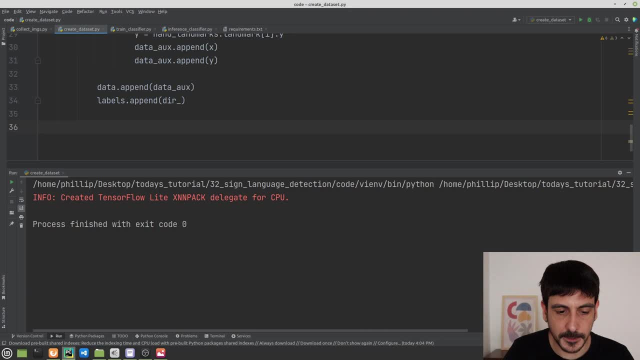 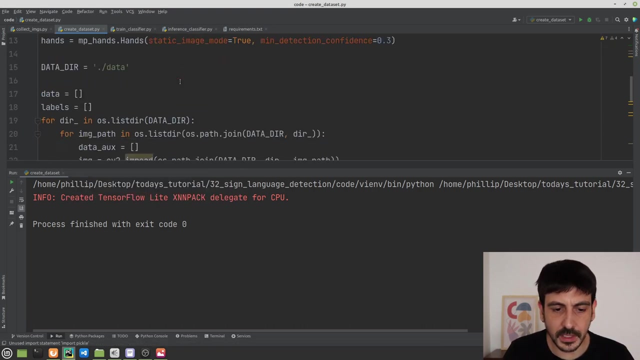 save all this data. so i'm going to do something like this: i'm going to define an object which is f and this is open data- dot pickle, if i'm not mistaken, i haven't imported pickles. i'm going to import it now. remember, pickle is a python library which is very commonly used for this. 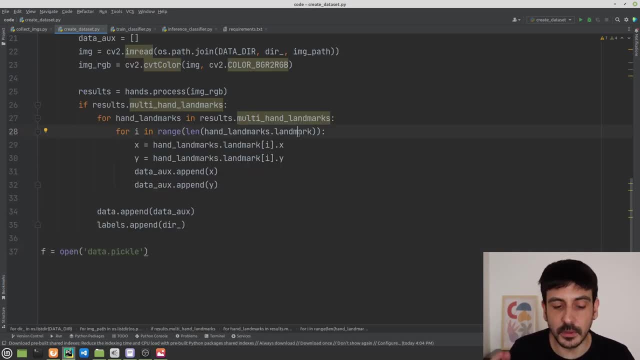 type of situations. to save data, to save you data sets, models and so on. it's just like a way to save this information. so we are opening this file and we need to do it like this. okay, because we are writing and it's also we are doing it as bytes, so we need to do it like this. then we need to say pickledump. 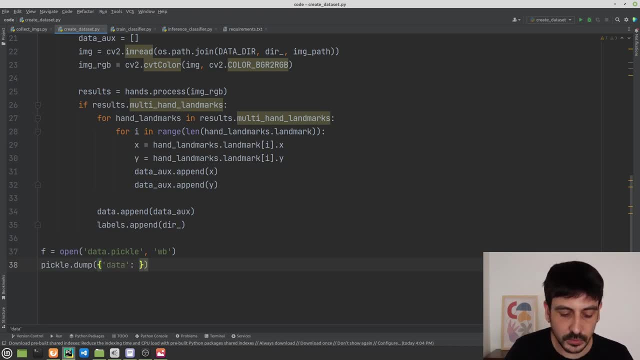 the object we are going to save and we are going to create a dictionary containing these two keys, and here we will have the data and the labels we have just generated, and then we need to close the file and that's pretty much all, and also we need to input f. 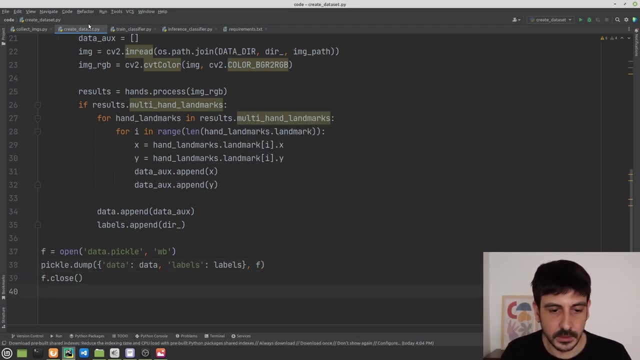 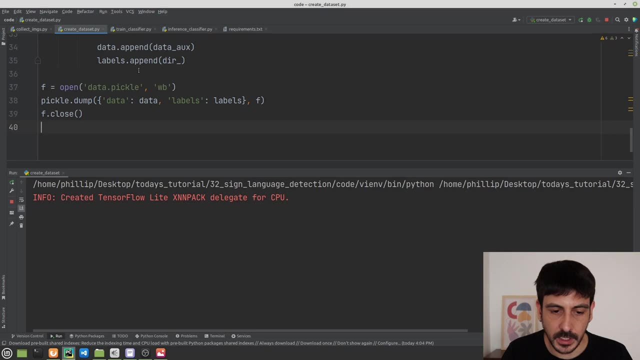 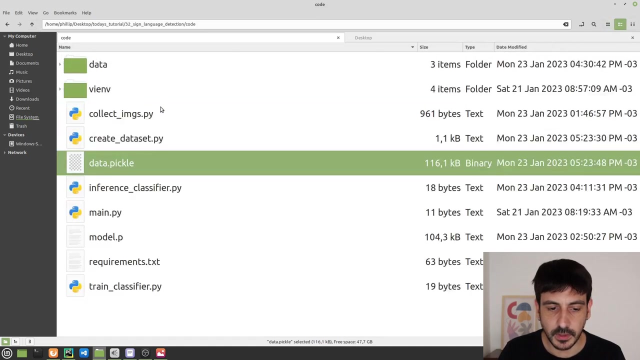 here and that's pretty much all. so let's see what happens. i'm going to run this again and, if everything runs successfully, we should have a file with this name. okay, everything runs successfully. now, if i go to my directory, i should see this file, which is the: 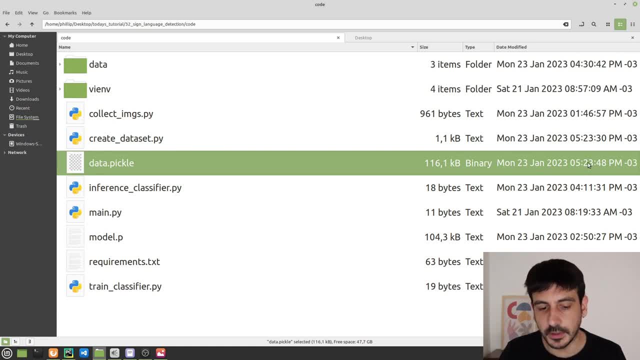 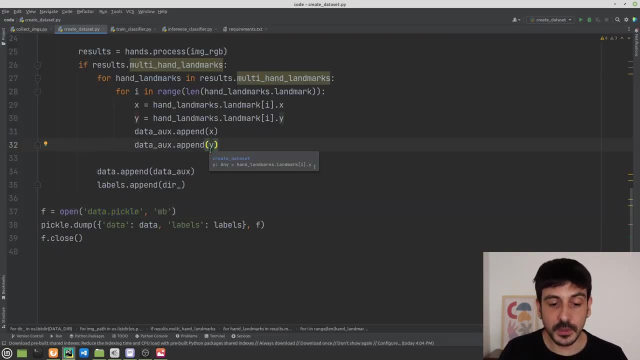 file i have just generated. you can see this is my current time, so this is the file i have just generated, and i have other files from our iterations or for executions where i was preparing this tutorial, but this is the file i have just shared. so, going back to pycharm, so everything. 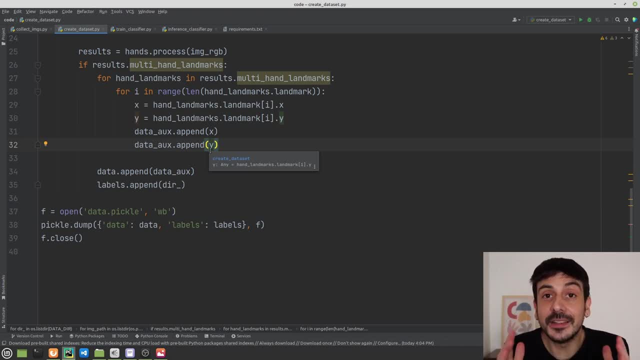 seems to be ready. for now we have created the data set. we are going to see some changes here in this data set. this is the data we are going to use in order to train our classifier, and now we can just continue to the next step, which is training this classifier. now we are going to take the data. we 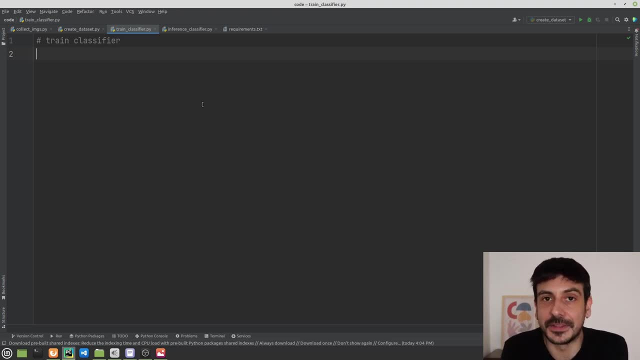 are going to load this data and we're going to train a classifier with it. so we are going to do exactly the same as we are doing here, but we are going to load the data instead. so i am going to import pickle, i'm just going to remove this train classifier and i am going to call pickleload. 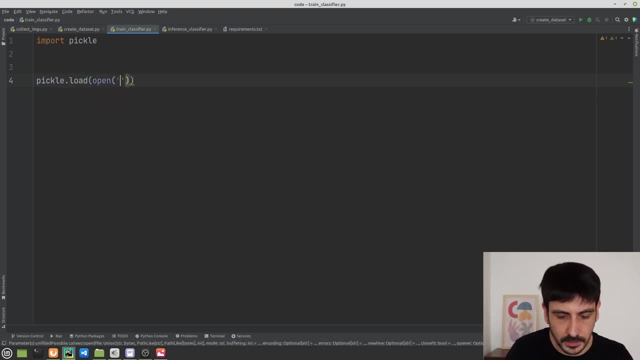 and this will be open, the file name, which is datapickle, and then i need to read this as rb. okay, and this will be our data file, or our data dictionary i, if i'm not mistaken. this is the way to read the data, and now let's print. 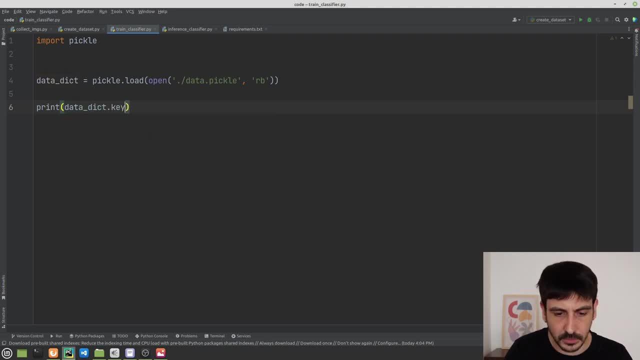 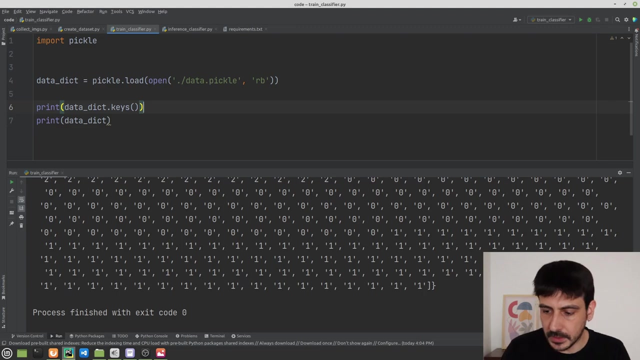 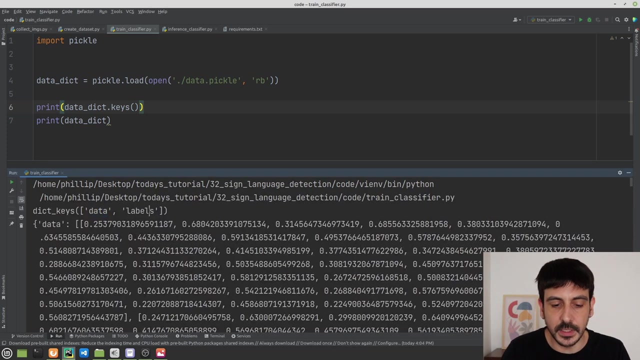 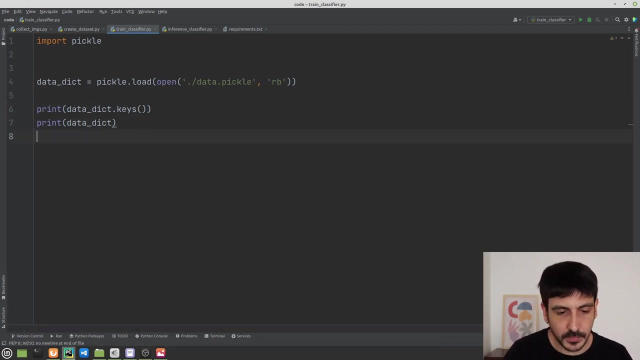 let's print two things: the keys of this dictionary and let's also print the object data- sorry, data dictionary. and let's see what happens. okay, everything seems to be okay. these are all of our labels and these are the dictionary data. these are the keys, data and labels. and then everything seems to be working properly. so now let's continue and 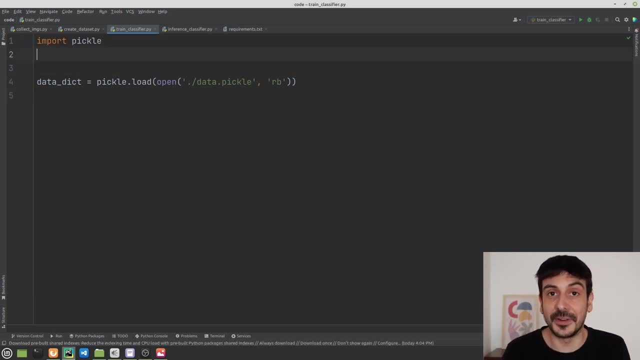 let's continue by importing all the different objects and all the different libraries we are going to use in order to train this classifier. we are going to train it using the library secret learn and we are going to use a very specific model, a very specific type of classifier, which is 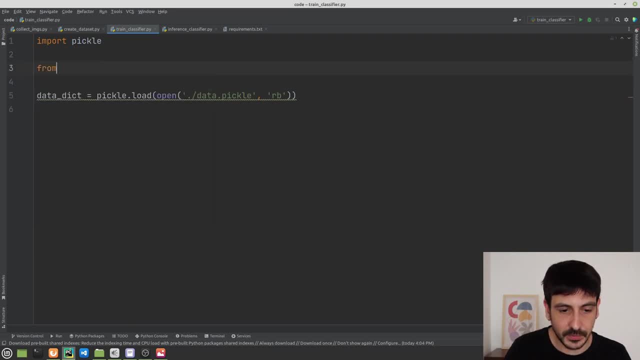 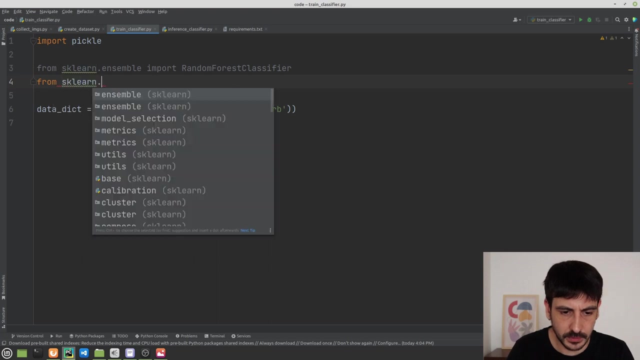 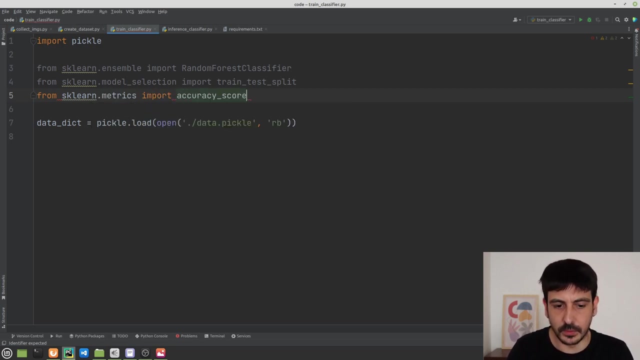 random forest. so let's start by importing from sklearnensemble: import random forest classifier, and then we are also going to import sqlearnmodule selection. import train test split, and we are also going to import from the metrics library accuracy score. okay, so these are the three libraries we are going to use. 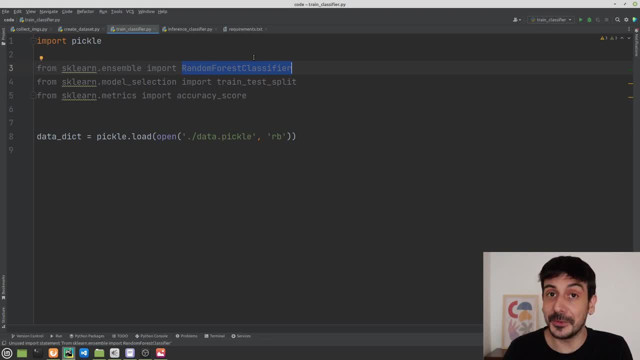 in order to train this classifier. we are going to train a random forest classifier, and these are two other functions we are going to need too. so let's start by unwrapping the data and the labels, and this is how we're going to do it, and we're going to call that a dict, and this will be. 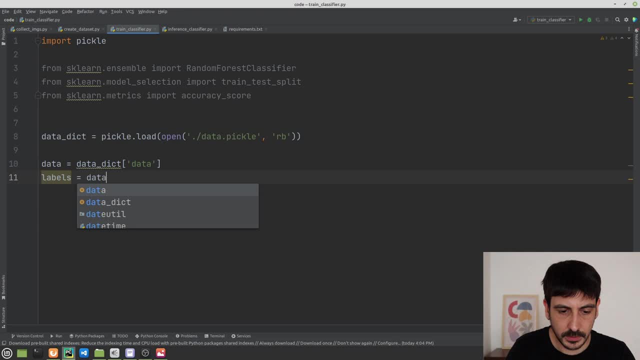 data and labels. data dict- labels- okay, and we need to convert this into a numpy array. that's all right. i need to import numpy too. i'm going to do it just now, because we just need to import it, because this is the way this classifier works, and 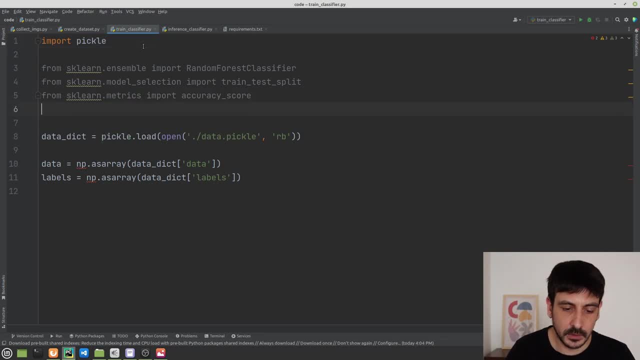 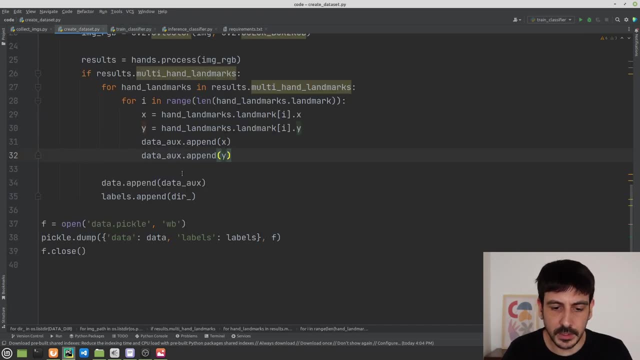 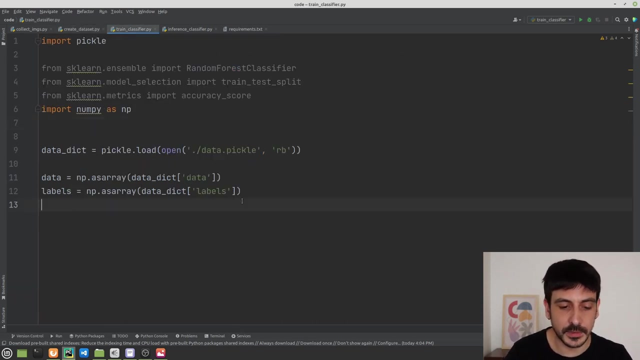 this is the way all these libraries work, so i'm going to import numpy as mp. remember that currently our data is as a list, right data and labels are lists. that's why we need to convert them into non-prs. okay, and the first thing we need to do in order to train this classifier is to prepare the data. 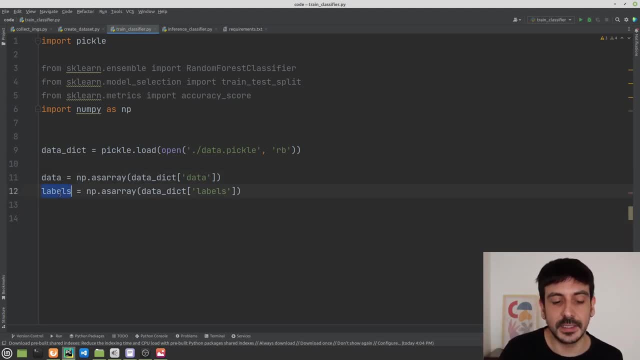 so we have all four data into these two: objects, data and labels. now we are going to split this data into a training set and a test set. this is a very common practice. when we are training a classifier- any type of classifier- we usually need two sets: a set we are going to use in a classifier. 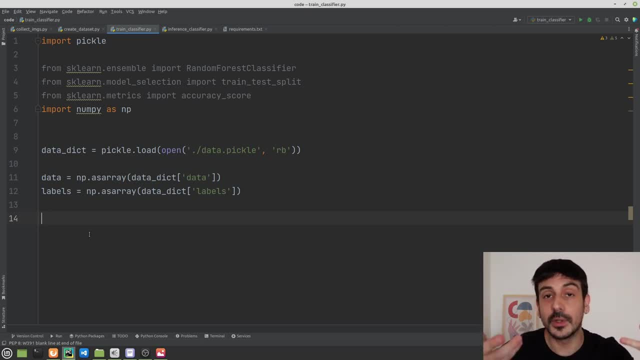 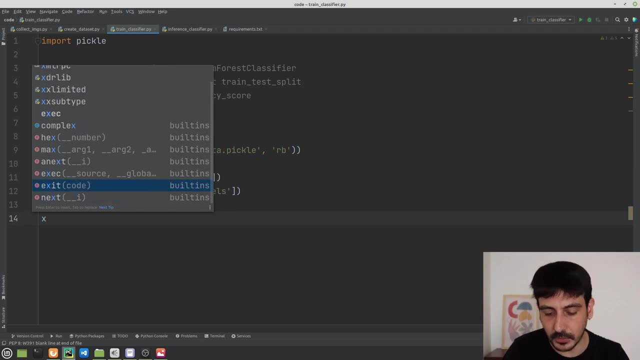 we are going to use in order to train this algorithm, and then another set we are going to use in order to test the performance of this algorithm. so this is what we are going to do and this is, uh, how we are going to name this training set and this test set. um, we are going to let me. 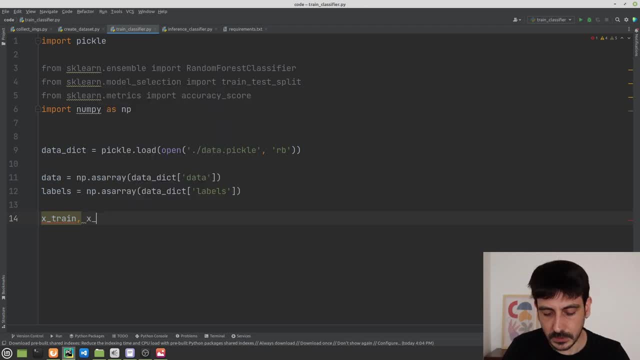 write this first and i'm going to explain it a few minutes. this is something like this: this is where we're going to use this function. we're going to input data labels. i'm just going to write everything down and i'm just going to explain it in a few minutes. um so, just bear with me, shuffle it through. 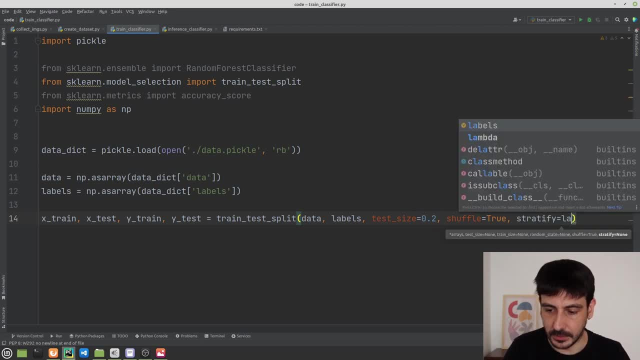 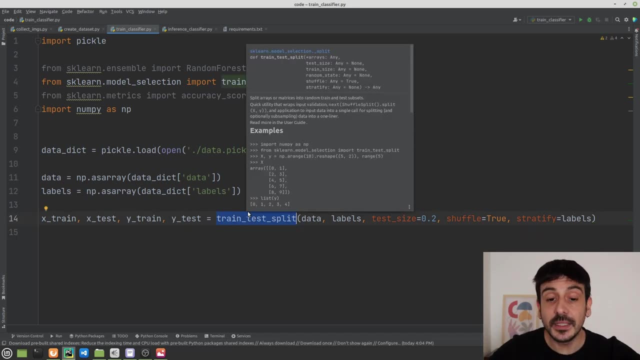 and then stratify according to labels. okay, so what we are doing here is calling train test split and we are splitting all of our data. we are splitting all these arrives and all this other array into two sets. right, so, from the data list, from the data array, 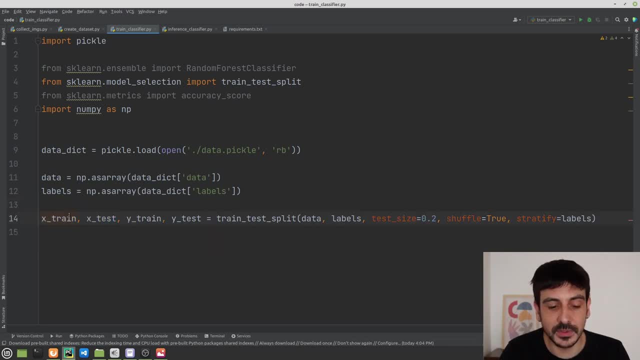 we are creating these two sets and you can see that one of them is called train and the other one is called test, and we're doing exactly the same for the labels. we are creating two objects, two arrays. one of them is trained and the other one is test. so we are taking 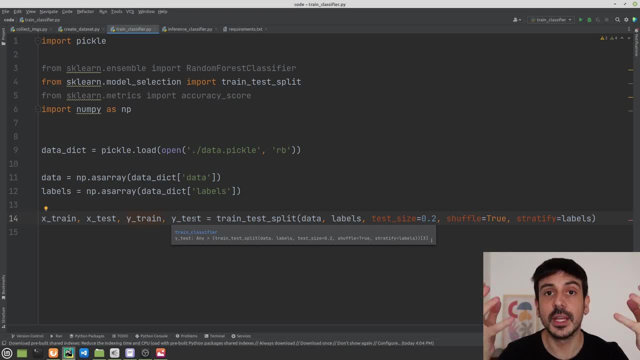 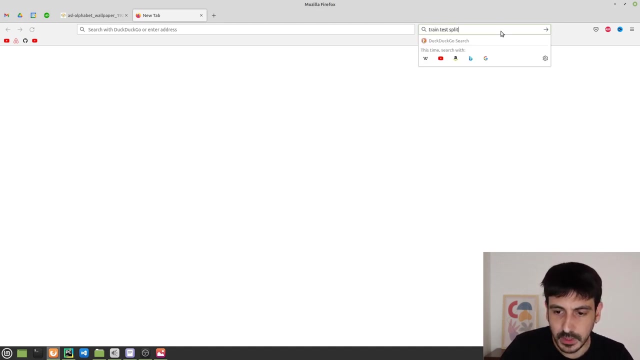 all the information within data and labels and we are splitting this information into two different sets. um, let me find a picture so i can explain this a little more. so this will be a little more clear. train test split. i'm sure we're going to have. we're going to find many, many different pictures. 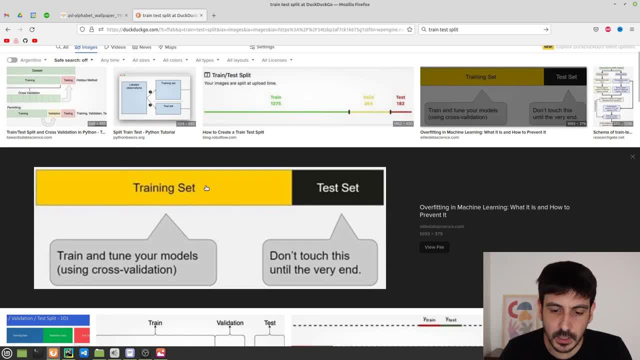 explaining how this is done. you can consider this image. so we have the entire array, the entire data, and we are splitting this data into two sets: training set and test set. so the training set is what i have called x train and the test set is what i have called x test, that's. 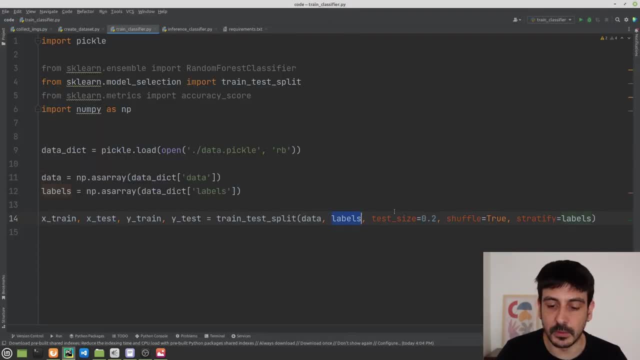 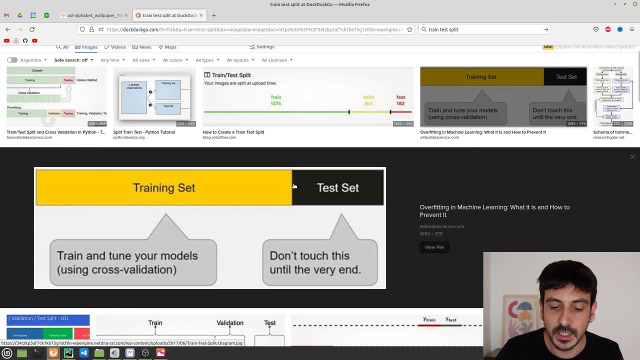 basically what we are doing, and we are doing exactly the same process for data and labels. then test size is the size of the test set. you can see that we have two sets and we can define the size of this test set for with different sizes. right, we could say: this is the 10 percent. 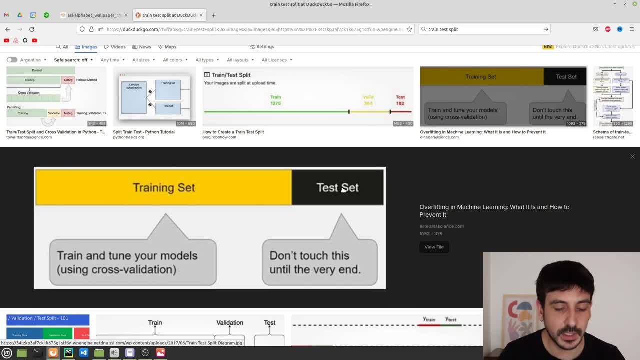 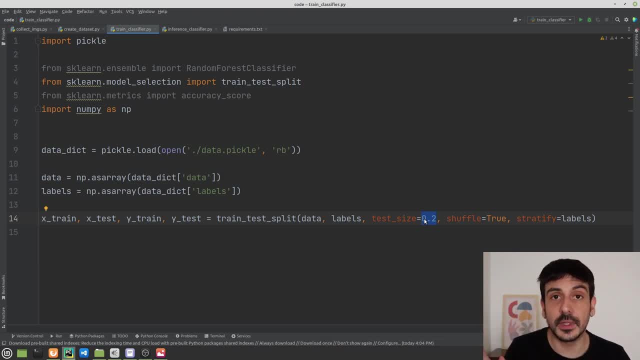 of the data: the 20 percent, the 50 percent, the 80 percent and so on. so i have specified this value in 0.2, which means we are keeping the 20 percent of our data, only the 20 percent as our test set, and 20 percent is a value which is very commonly used as a test. then shuffle equal true means we 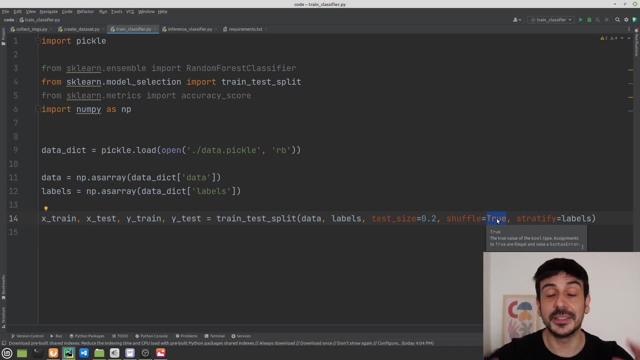 are shuffling the data. this is a very good practice, it's a very common practice and i will advise that you always, always shuffle your data when you are doing something like this, when you are training a classifier, because this is something i have mentioned- i have covered in other tutorials where i also show you. 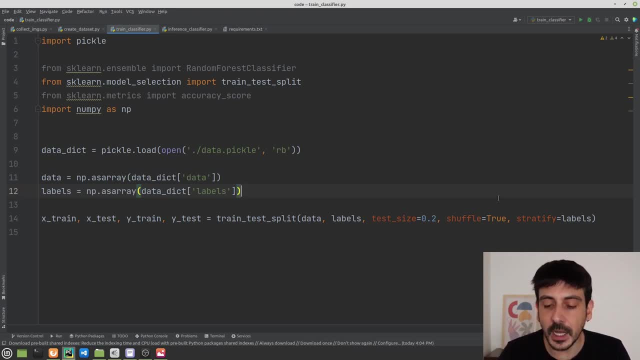 how to train image classifiers or different type of classifiers, and sometimes there are different biases in our data that we are not aware of, so shuffling the data is a very common practice. even when we think it's not a long story short, always remember to shuffle the data. 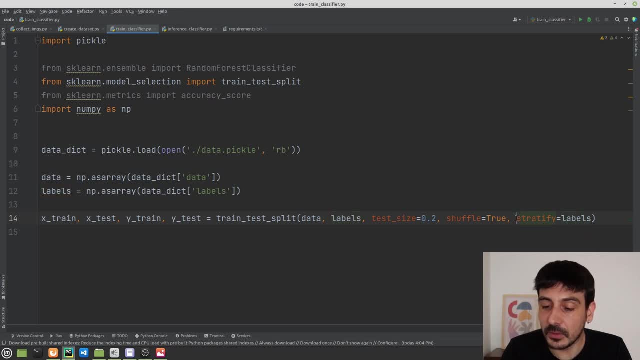 it's a very common practice and i will advise that you always shuffle your data when you are training a classifier, because it's very common practice even when you are training a classifier. so, after you built your database, it's very important to keep the tables and 우 mw is. 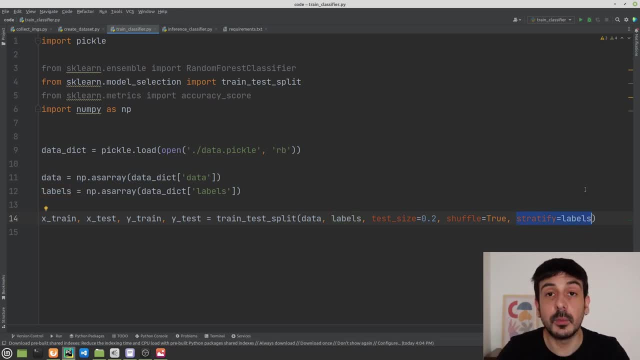 going to be much, much better then. stratify equals labels. this means that we are going to split the data set, but we are going to keep the same proportion of the different labels, of the different categories we have in this object. we are going to keep exactly the same proportion in the 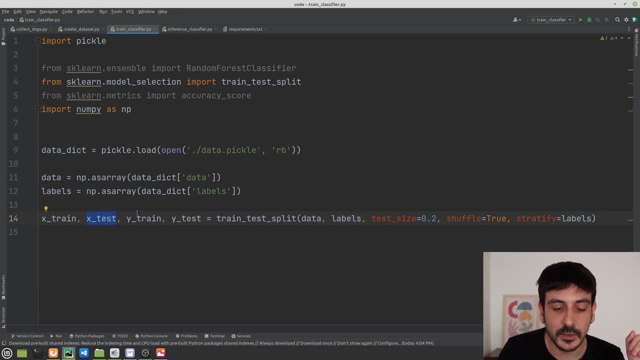 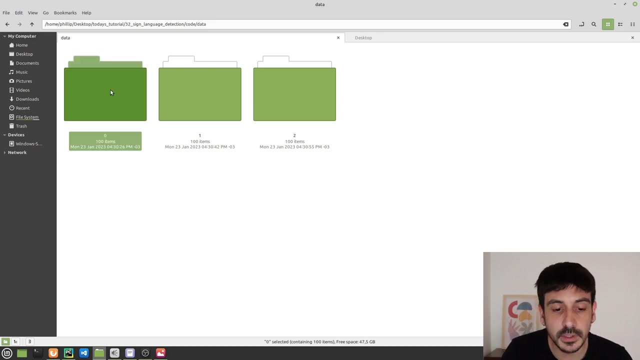 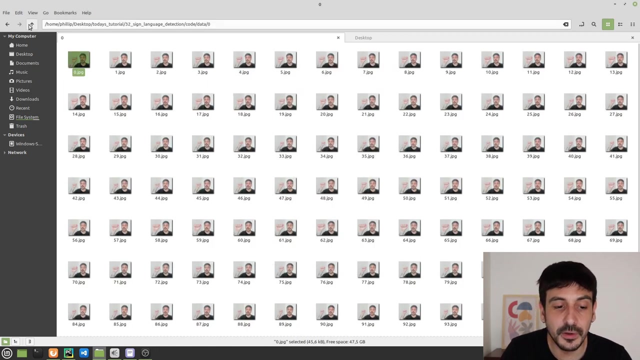 train set, as in the test set. right, so this object and this other object are going to have the same proportion of all of our different labels, right so? so we are going to separate the data into two. So, if you remember the data we are using, we have 100 elements in this category, 100 elements in this other category and 100 elements here. So this means that one third of the data is labeled as A, which is this symbol. One third of the data is B and one third is L. 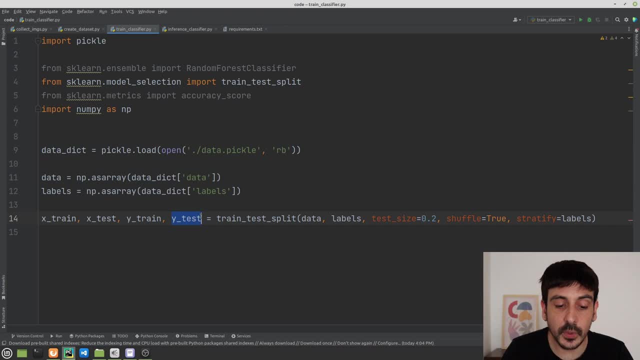 And if we look at these two objects, white train and white test, we are going to see exactly the same proportion. One third of all the data, of all of the elements in this array, are going to be A, then another third will be B and another third will be L, and exactly the same situation here. 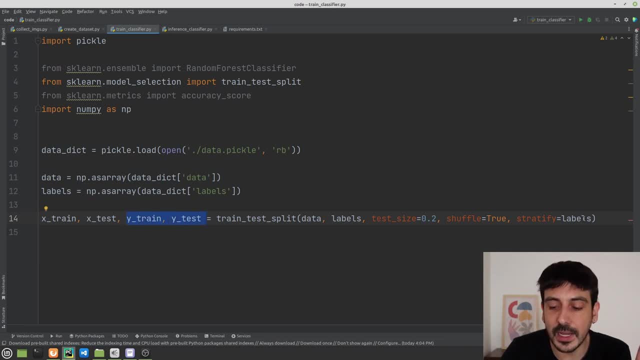 So that's basically what it means when we are stratifying according to the labels, And that's also a very common practice and a very good practice when we are splitting a data set. So always remember to include stratify equals labels when you're using train test split. 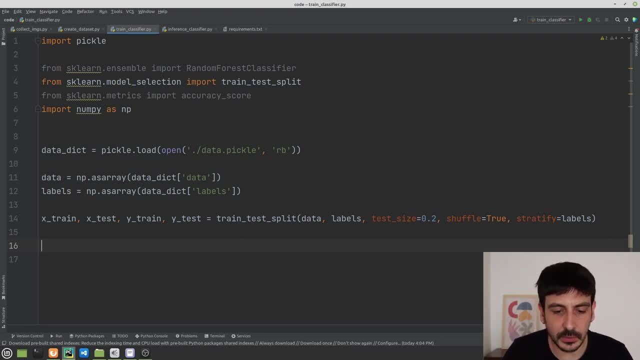 So this is all for splitting the data, And now it's time to create our model. So the model we're going to use, remember, is a random forest classifier. So this is a classifier we are going to use And the first thing we need to do is to train this classifier. So we are going to call fit, we're going to input X train and white train. 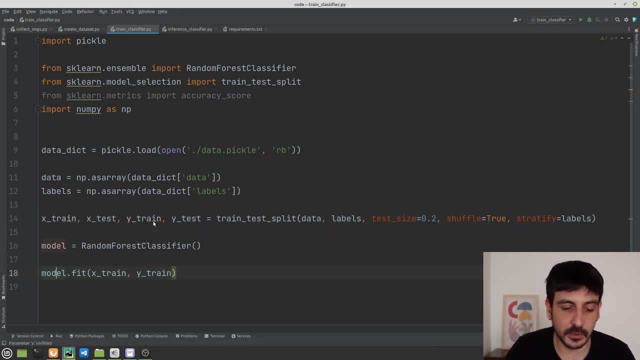 This is the way we are training this classifier, This is the way we are fitting this model, And then we just need to call dot predict, And we need to input X test, And this will be Y predict. And that's it, In only a couple of lines. we have trained the classifier and we have also made our predictions. 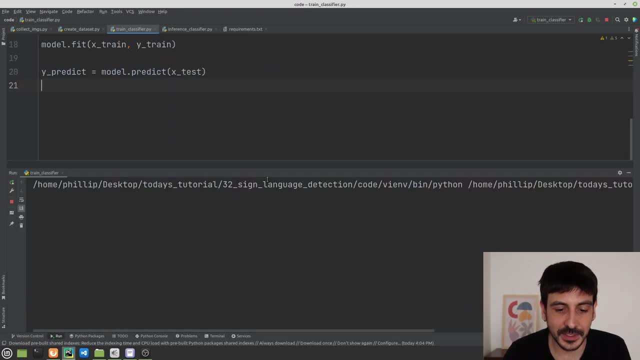 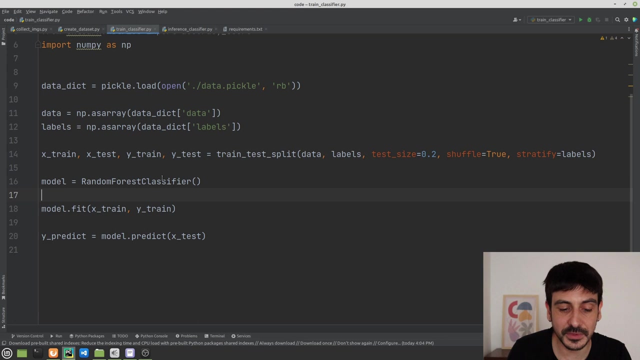 This is how simple this is. So let's just execute this script to make sure everything works properly. Everything works properly And you may notice how fast it was right. This took only a few seconds. If you are familiar with machine learning algorithms, with training machine learning algorithms, you will know that sometimes it takes a lot of time to train a classifier. 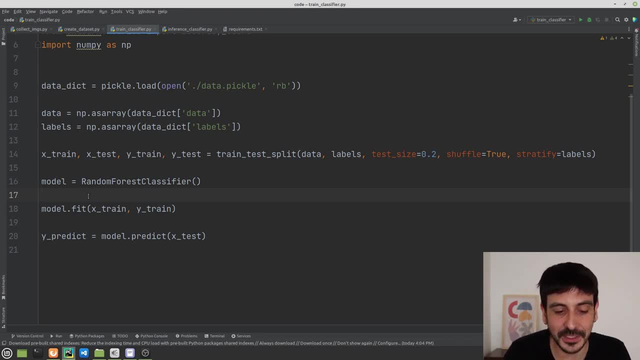 But in this case this is a very, very fast training. So that's one of the reasons I chose random forest: because it's like a very simple algorithm. I know the training is very fast. I know that it's robust enough for our problem, for our project. 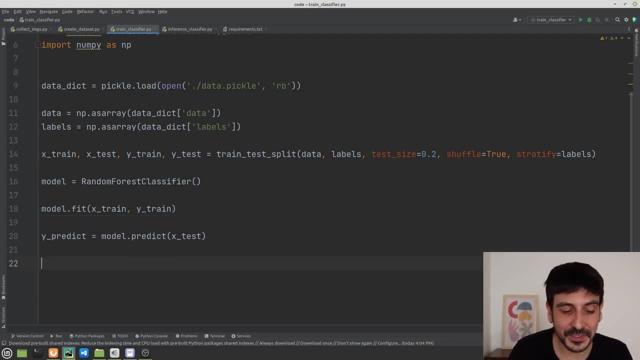 So we have already trained the classifier, We have our predictions And the only thing we need to do now is to see how this classifier performs. So I am going to find a new variable, which is score, And this will be accuracy score. 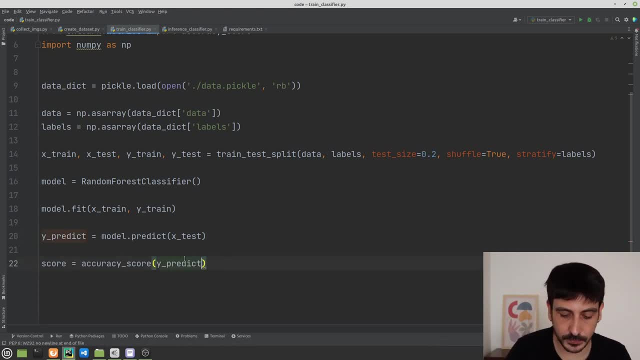 And I'm going to input our predictions, And then I'm going to input Y test, which are our labels, And now I am going to print: Okay, And this will be something like I'm going to express it as a percentage of samples were classified correctly. 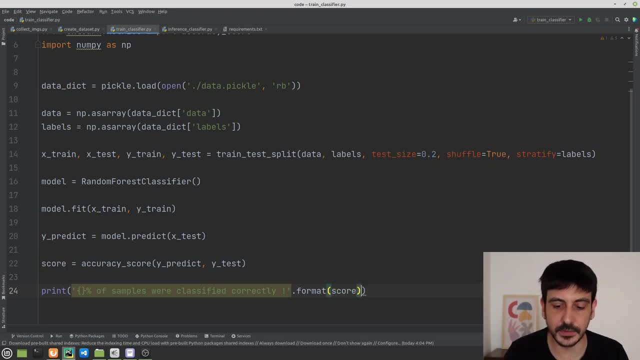 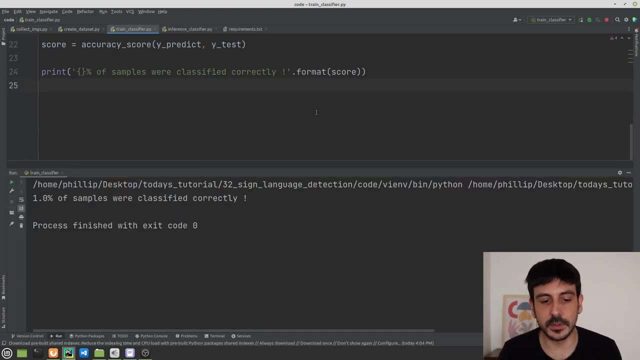 Format And this is something like score, something like this: Let's see what percentage of our samples were classified correctly. So I'm going to run this code And you can see. oh, I forgot to do something which is multiplying this value times 100. 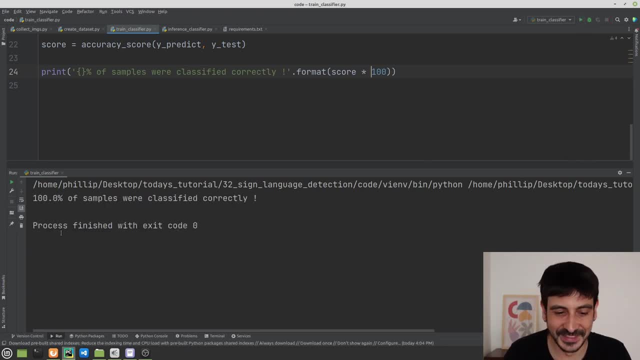 You already saw the answer, but anyway, let's do it again. 100% of our samples were classified correctly, So this is amazing. This means we have a perfect performance. We have trained a classifier with a perfect performance, So everything makes sense now. 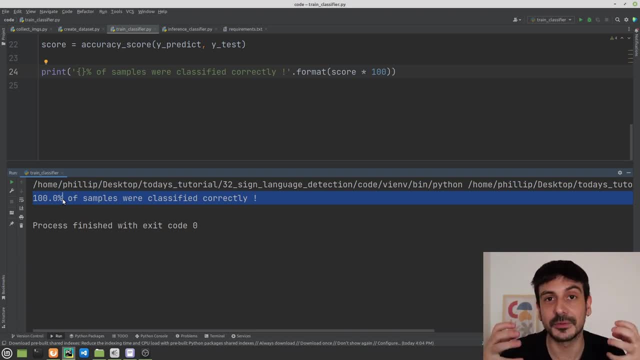 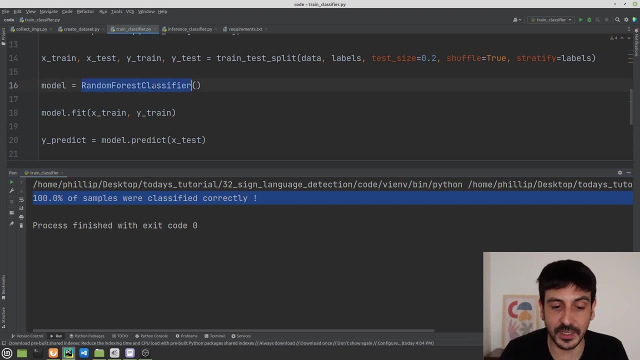 Okay, And now we are going to use the data in order to extract all the landmarks from our images, from our hands, because that's where we had all the information. And now the selection we did for this classifier because we had the intuition: this is not. 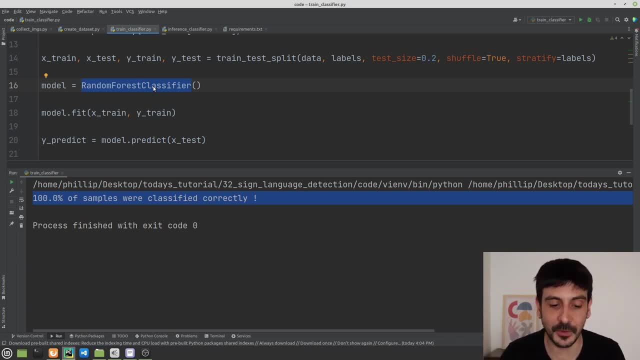 really a super, super complex problem, and a random forest will do just fine. Everything makes sense now, when we are achieving a 100% accuracy right. So this is very good, And the only thing we're going to do now is to 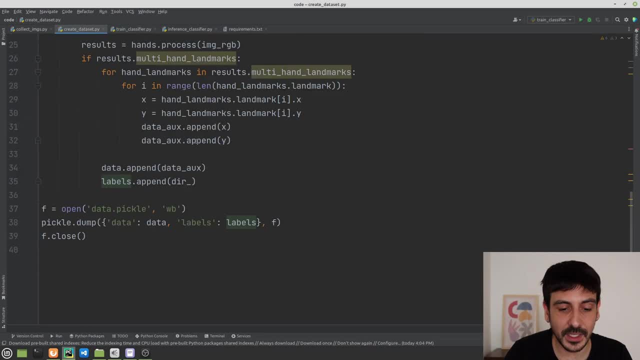 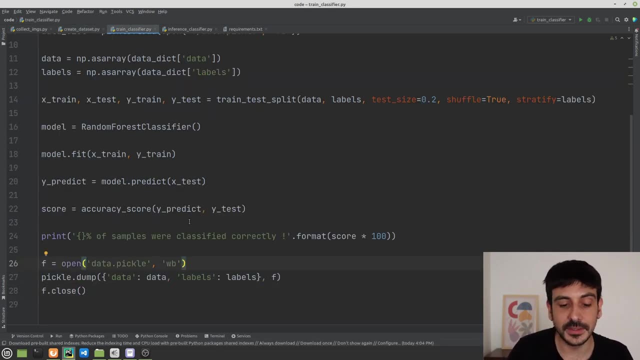 Save this model the same way we save the data here. We are going to save the model because we want to use this model later on to test the performance of this model, but not testing the performance as we did here, but testing the performance of this model with real data. I am going to, uh, make some gestures, some 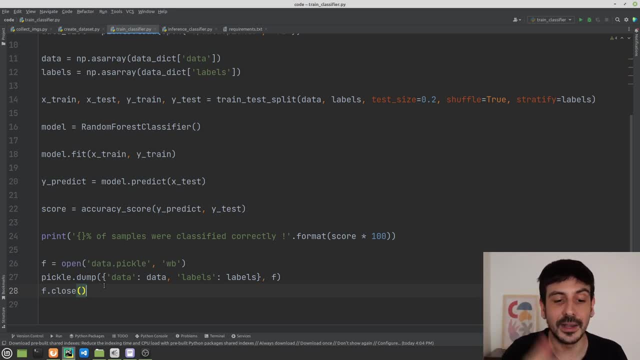 symbols and we are going to classify these symbols- uh, live on my camera on this video. So we definitely need the model, Okay, So I'm going to save this model like model dot P, and I'm going to do something similar. 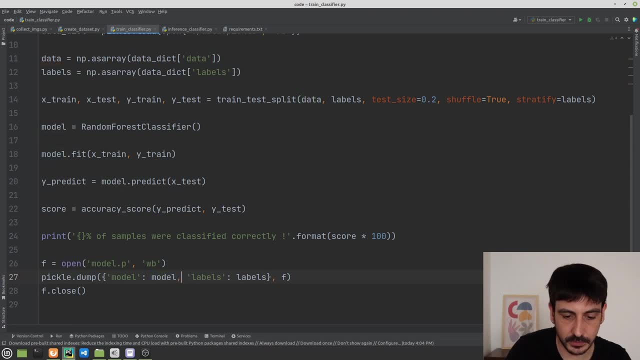 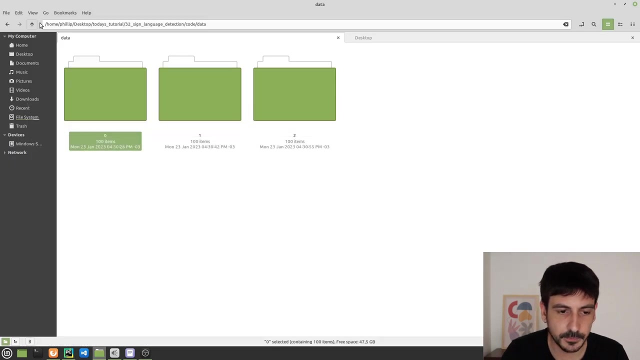 I'm going to say model- uh, this will be model, uh, this. okay, So I am saving a dictionary with only this object and I press play, and that should be it. We have to wait and then it's, it's completed. 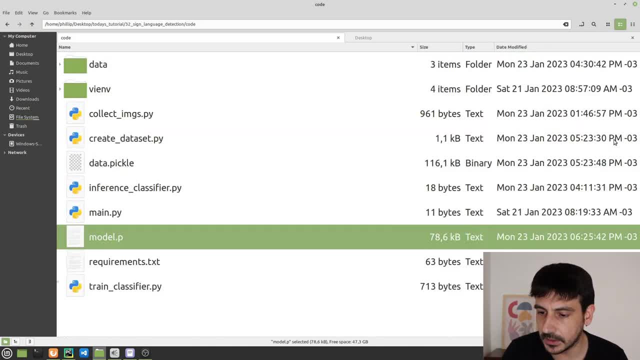 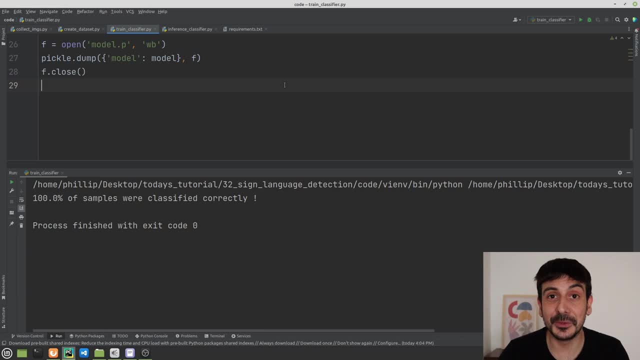 If I go to my directory, you can see the model we have trained is here and this is my current model, So that we should be fine, It's already done. Okay, So everything is almost ready, Only we we have only one step left, which is testing this classifier. 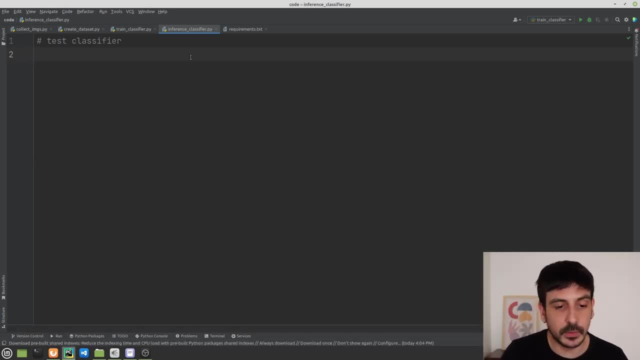 So that's what we are going to do now. Okay, Now it's time to test, or classifier, And the way we are going to test this classifier is by importing CV too, because we are going to access or welcome, and we are going to do all these different symbols in our weapons. 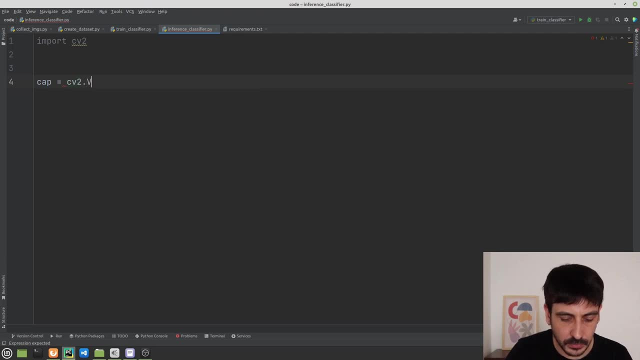 see what happens. so cap will be something like cv2- video capture, and i'm going to access this webcam- the number two- and then, while true, uh, cap dot read, uh, this is red, and frame. and then i am going to call cv2, im show, i'm going to call this window frame and this will be my 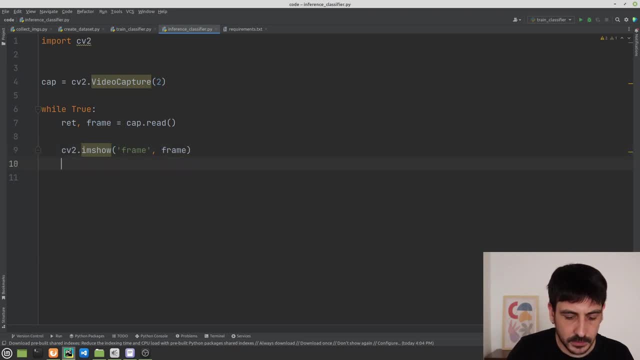 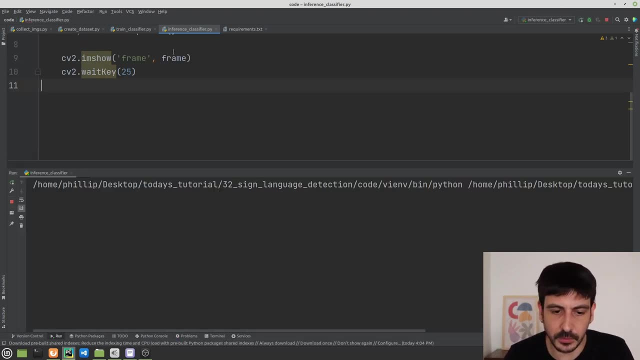 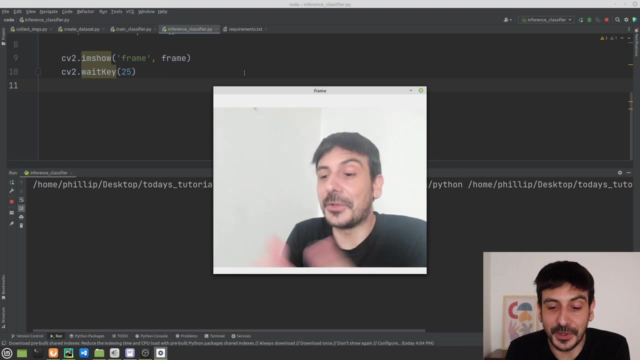 frame, and then cv2 weight key, and here we should pull a 25, which means we are going to wait 25 milliseconds between each frame. right? so everything seems to be working fine, and this is my webcam. so, um, what we are going to do now is we are going to detect all the landmarks. 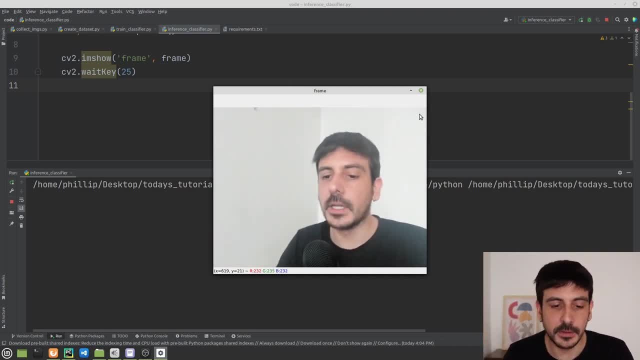 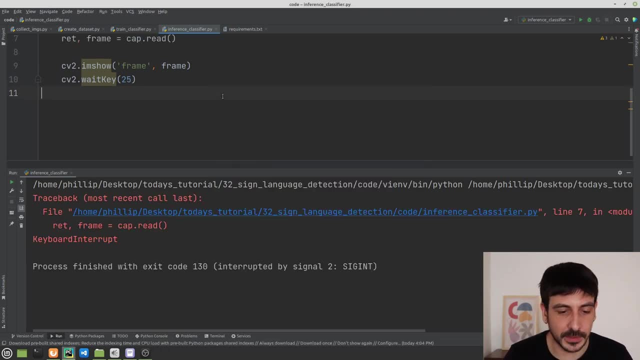 in this webcam, we are going to detect all the landmarks of my hand, and then we are going to use the classifier we just trained in order to know what a symbol i am displaying in my hand. so let's do that. i am going to release memory. i'm not sure if it's. 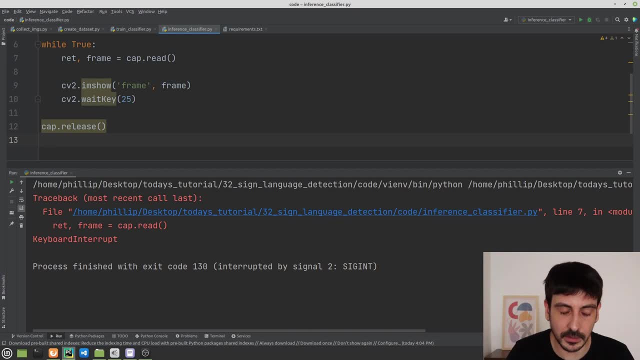 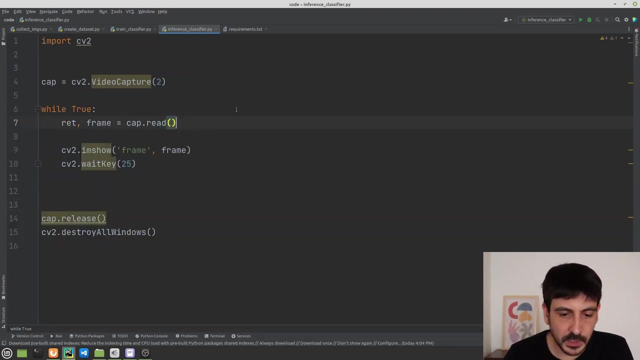 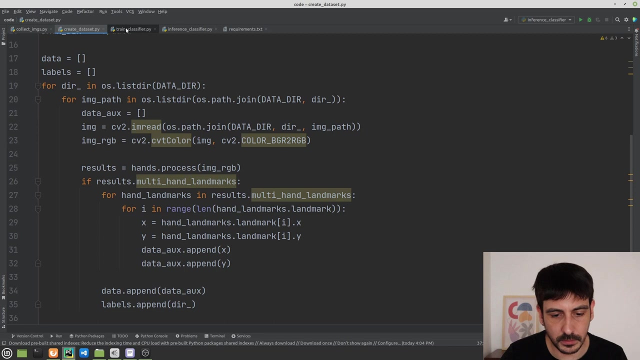 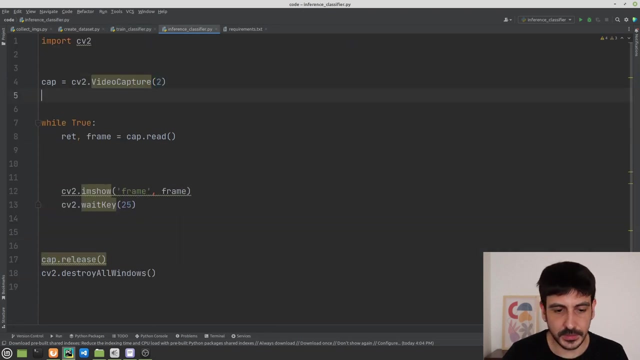 really new because we are exiting the program- the program anyway- but i'm going to do it just just because it's a good practice. cv2 destroy all windows and that's pretty much all. so i don't have much space here, so let's go here and i'm going to copy a few objects. i'm going to copy this, which is the um. 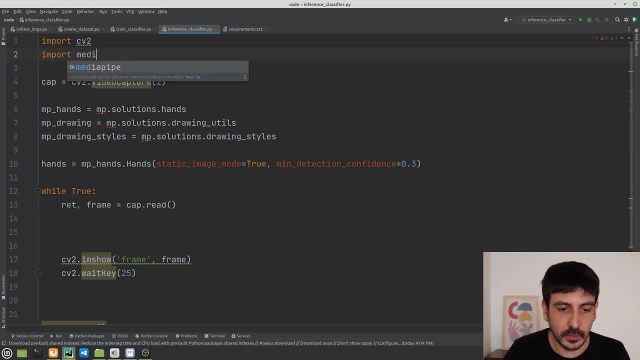 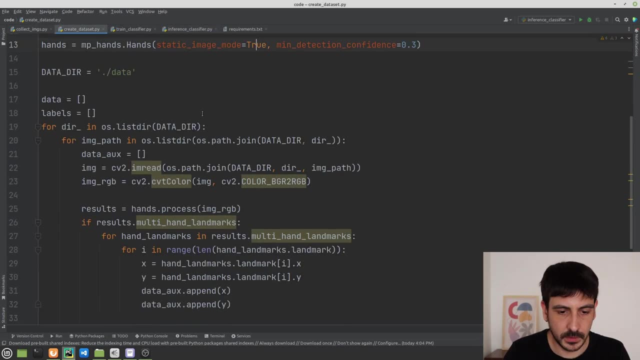 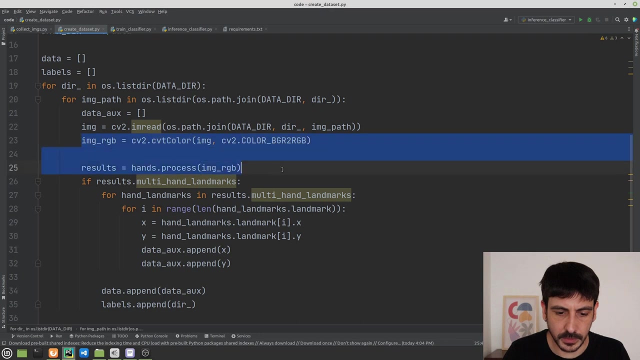 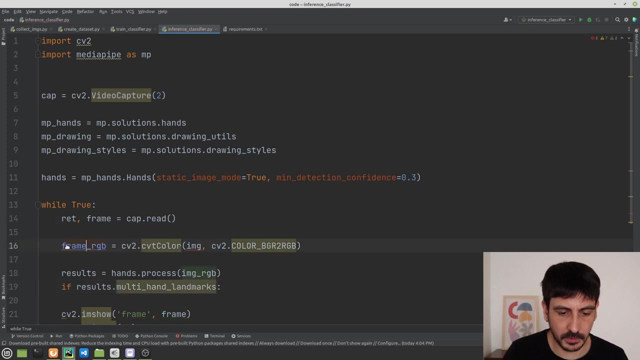 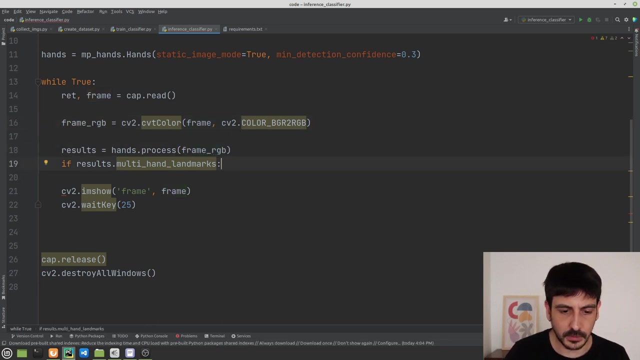 the media pipe library or the media pipe functions we used, and then i am going to. we also need the color conversion, but i'm going to do this. okay, something like this: this will be frame rgb, frame, frame rgb, and this is where we are going to um go through all the landmarks and we're going to do something. 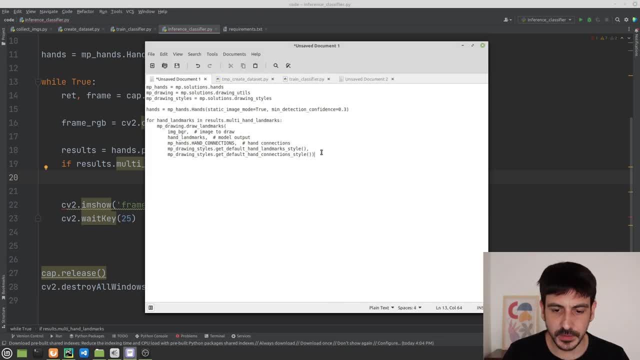 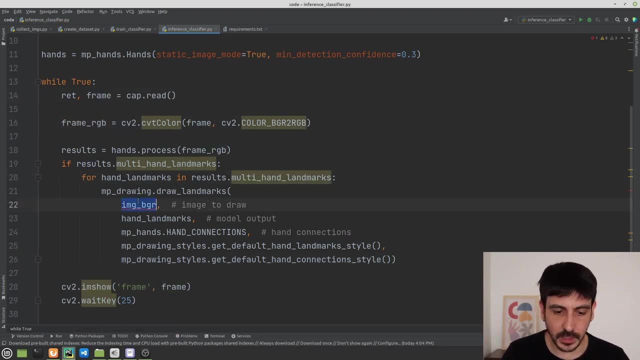 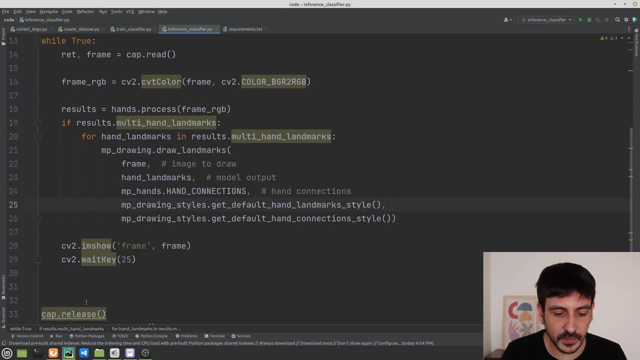 similar as we did before. so i'm going to copy this code i used before, and the first thing we're going to do is to draw the landmarks on top of the webcam and then we are going to classify it. so, as always, it's always a good idea to go one step at a time. 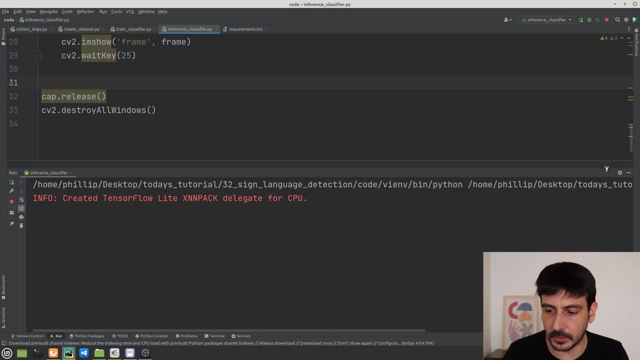 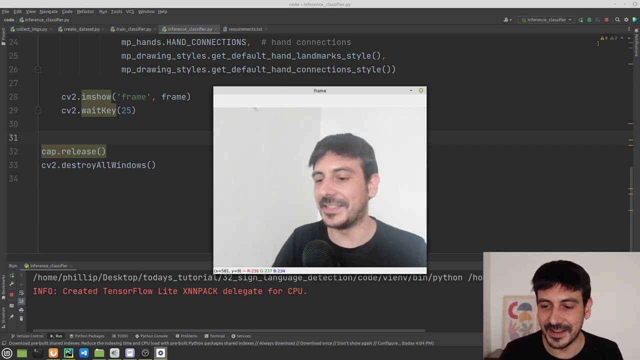 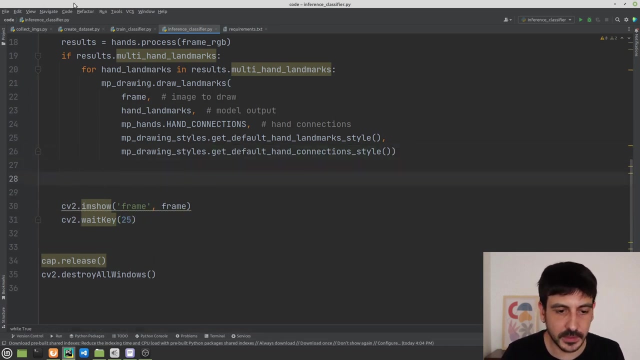 and let's just run this code to see if everything works properly. everything seems to be working properly. you can see we are getting the landmarks from my hand and now it's the time we are going to classify this object. so we go back here and we say something like this: we are going to iterate in all the landmarks. 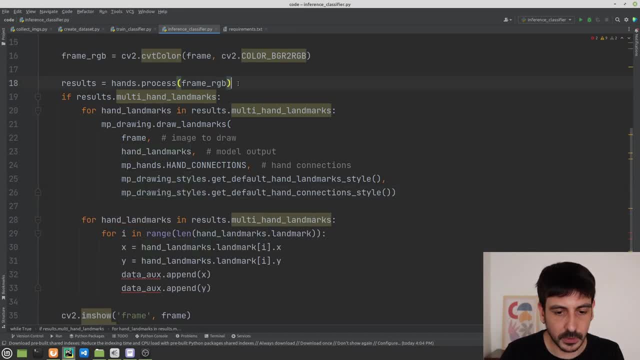 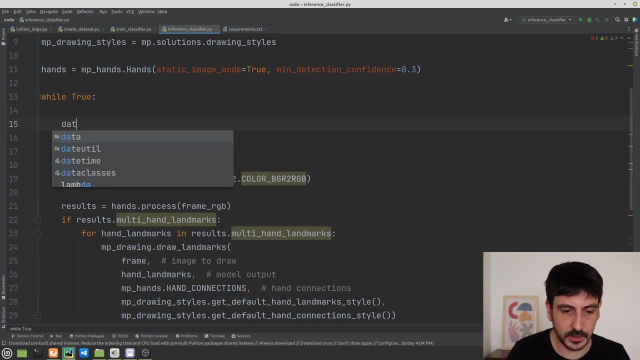 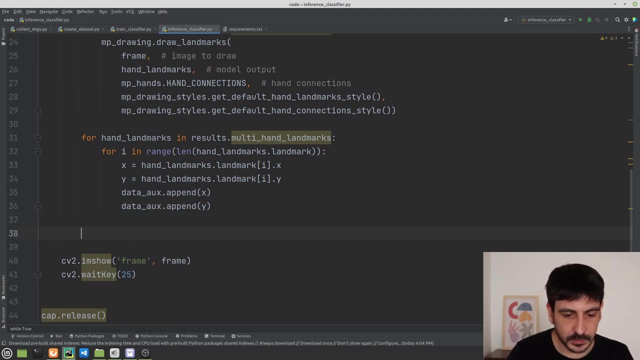 the same way we did before. and now we are going to create a, an auxiliary array, which is this: the same way we did before, and the only thing we need to do now is to use the model. but we need to read the model first, we need to load it. 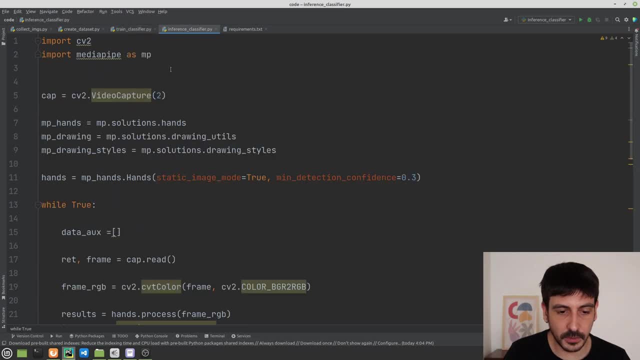 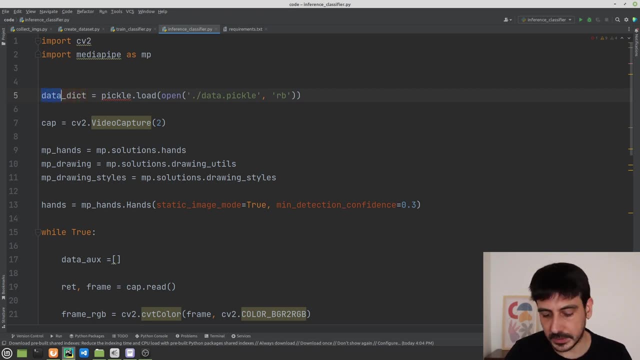 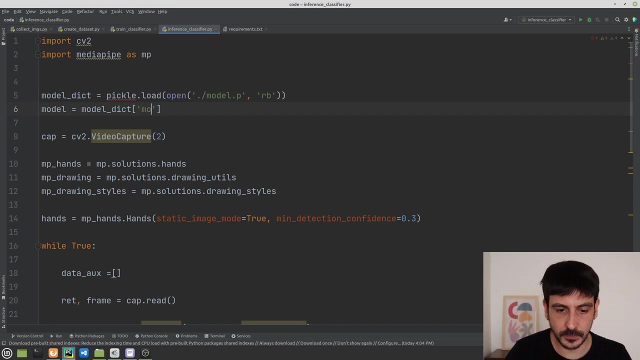 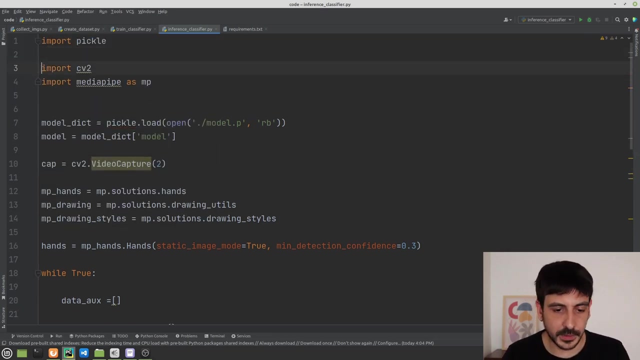 model first. so let's do something as we did before. i'm just going to define it here. let's say model dict is equal to pickle load, model dot p. and then let's say model equal to model, dict, model, and obviously i need to import pickle, okay, and this should be enough. now we are here. yes, we are here and we need to. 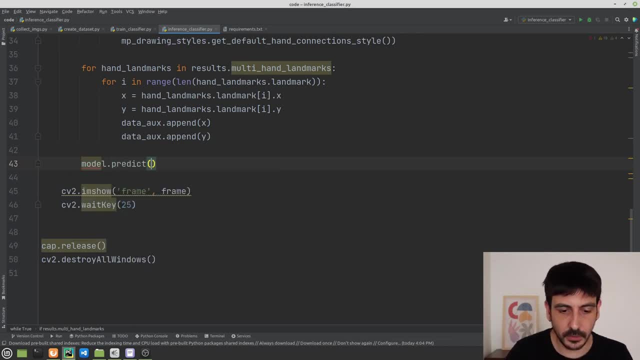 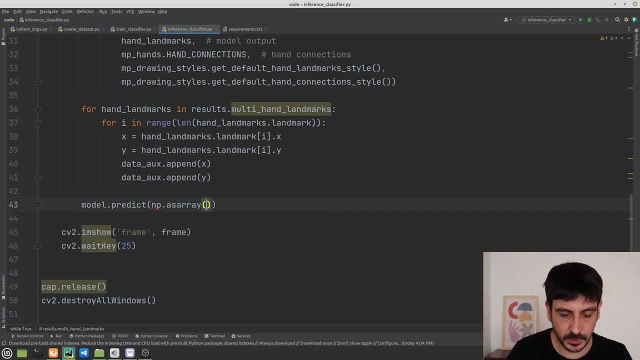 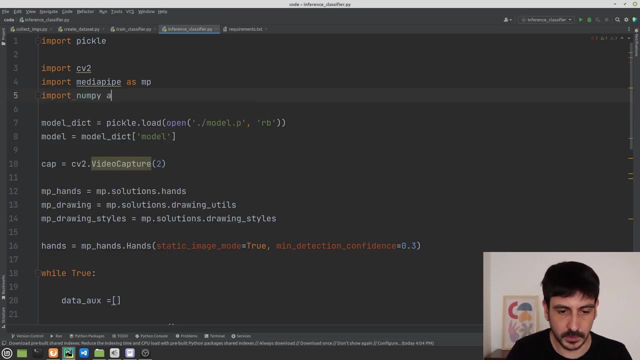 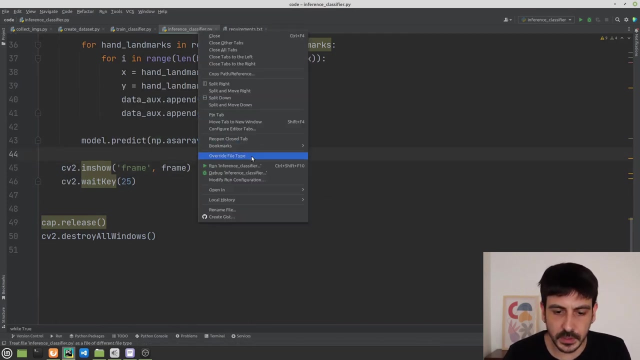 use model to predict the category. so let's see what happens. this will be mp as array from data out- okay, we need to import mp2 from data out, okay, and let's see. let's see what happens. let's see if we don't get any error. 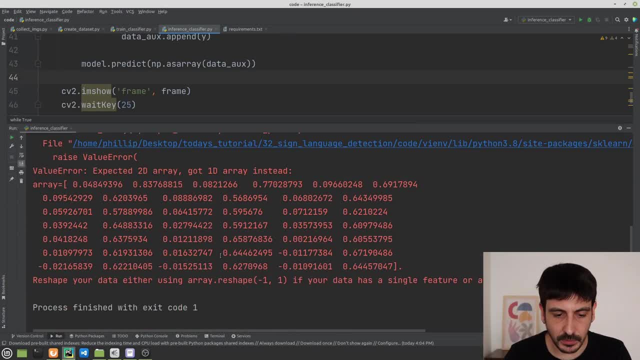 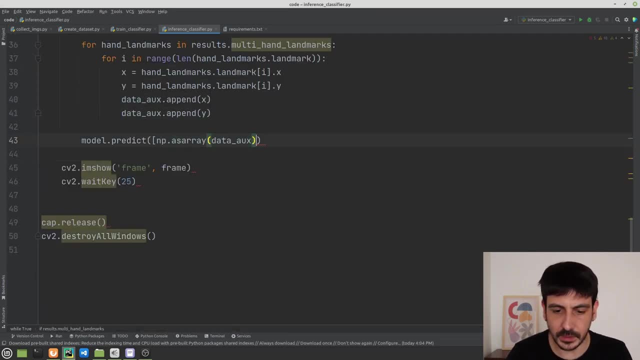 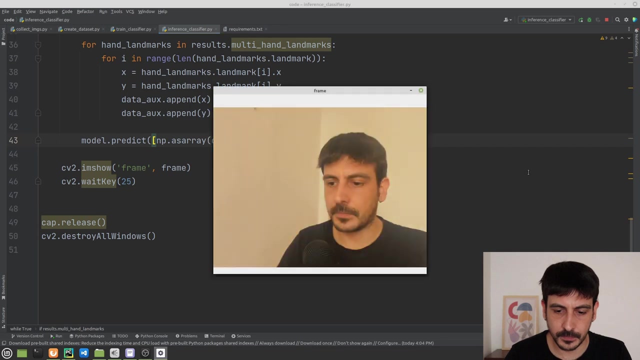 okay, we get an error, of course, and it's related to the shape, if i'm not mistaken. what we need to do now is to input this as a list. let's see what happens now. so it was not an error. yeah, everything it's okay. so now we are using our classifier in order to 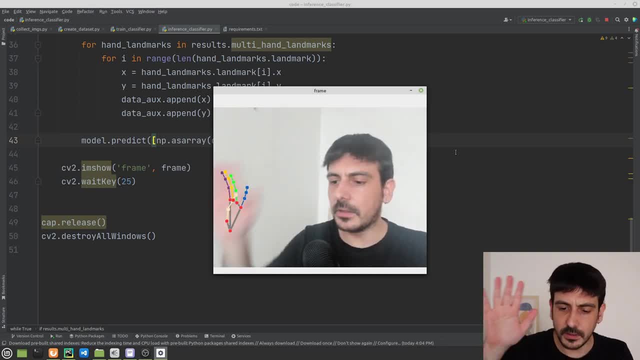 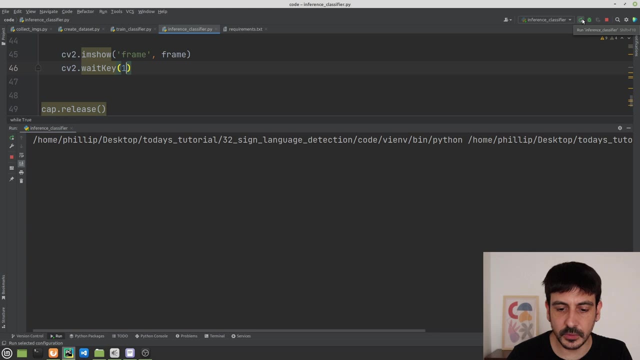 classify the uh class for these landmarks we are. we have like a very like a more poor performance now. now it's better. it seems the classification is not making this real-time. maybe if i do something like waiting only one millisecond, it's not like it's the most important thing, but and 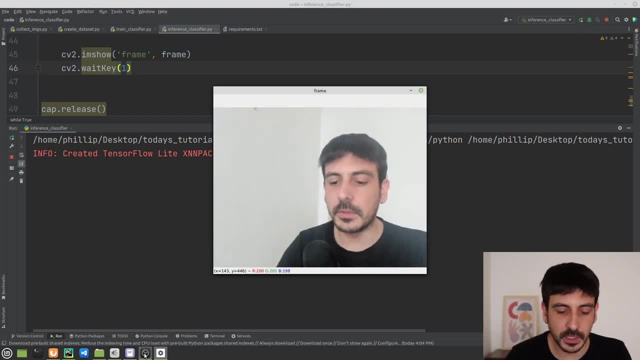 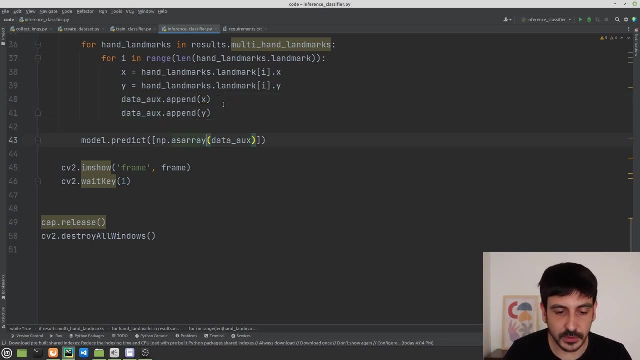 now it's a little better, remember, I'm also recording my screen, so that takes resources. that's pretty much the reason I think. so let's continue. everything seems to be working properly, and what we will do now, now that we have our prediction, this is our prediction. we are going to draw the prediction on top of. 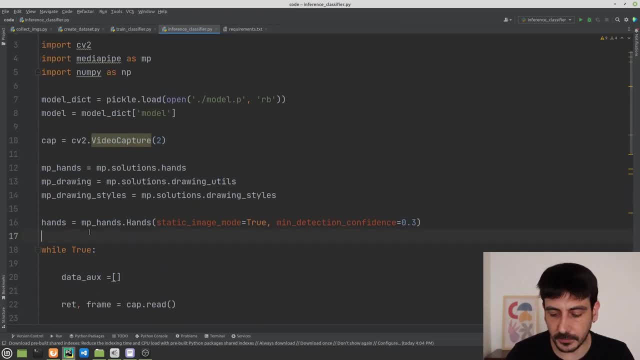 our frame, or actually what we can do. we can define a dictionary which is something like labels, dict. and this is 0, equal to a. remember the number 0 represents the a character, then 1 represents B and then 2- sorry, I'm doing things wrong- and 2 represents. 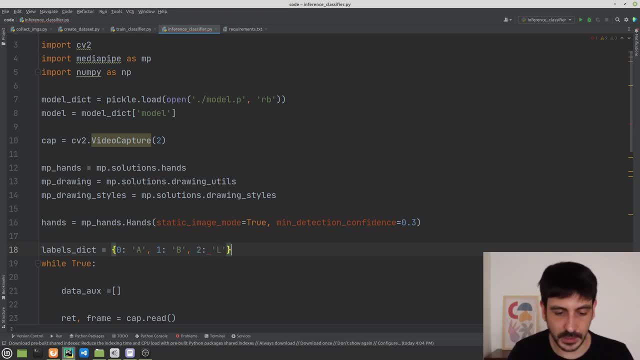 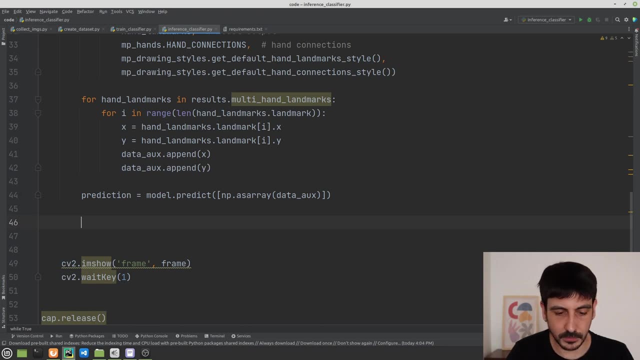 b and then 2- sorry, I'm doing things wrong- and 2 represents b and then 2 represents l. okay, and what I can do now? something like: predicted character. it's equal to labels. dict: int: prediction 0, because we are getting a list. prediction is a list of only one element, so we need to do it this way, okay. 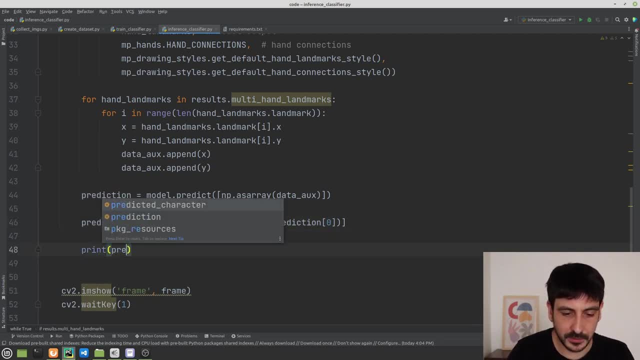 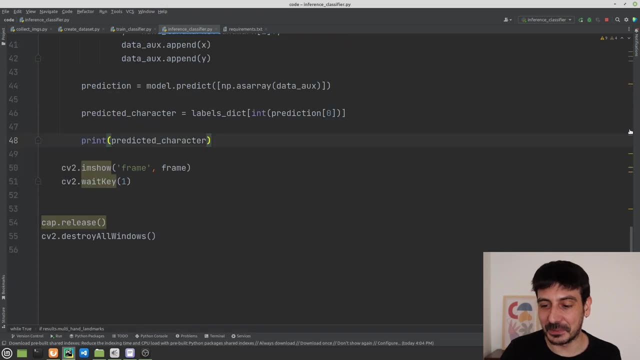 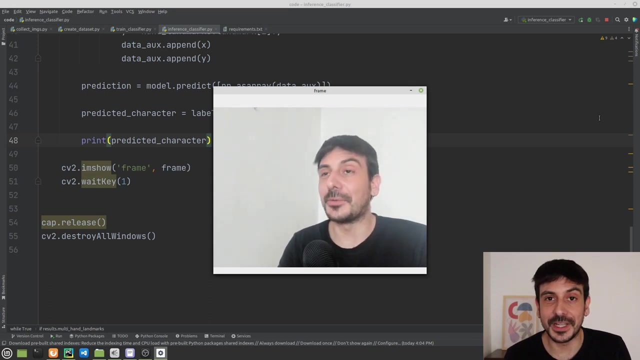 that's pretty much all. let's print predict its character. I'm super excited. let's see if this works. I'm super excited, so I press play and now let's see if we can accurately detect and recognize all the symbols we have just trained. so the first one is the a. I have to put my 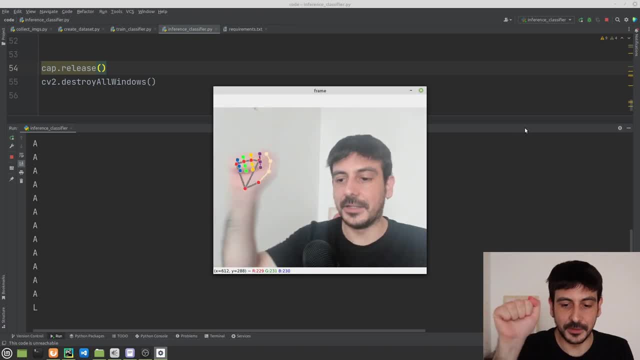 name in this value here, so that when I press this l, that means I have to do everything right. so let me just say, run again, and if I do the a character you can see I'm getting a. once and again I'm getting a. so everything seems to be. 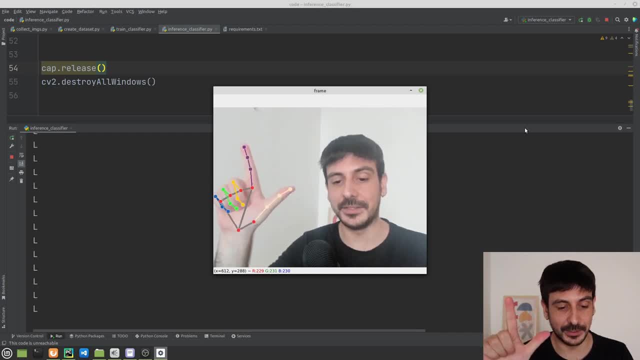 working properly. now I'm doing the B and you can see I'm doing, I'm getting B. once and again, I'm getting B and everything goes perfect. and if I do l, which is this value, you can see I'm getting the l and also the accuracy. it's perfect. so that's. 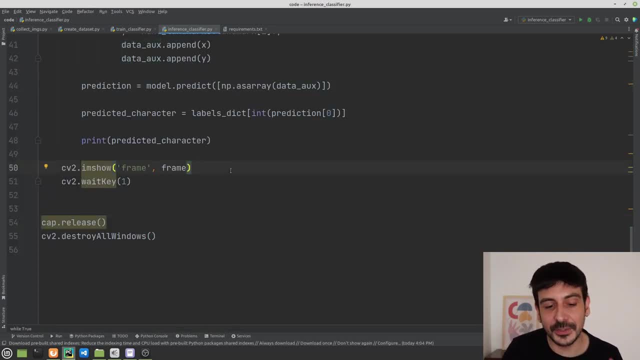 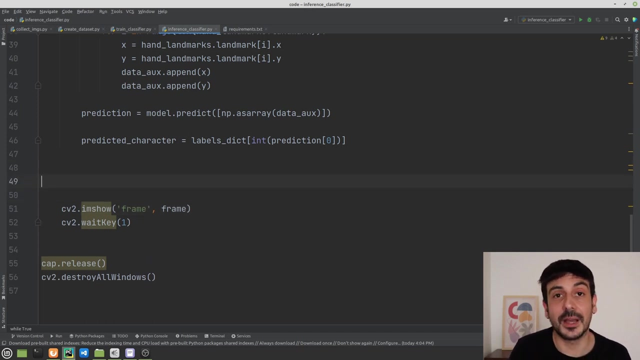 to do now is to make a more pretty drawing right. let's just print the um, the prediction, on top of the frame and let's do also like a bounding box, around the prediction around the hand we are detecting. so that's what we are going to do now, but you can see that we have solved the problem. 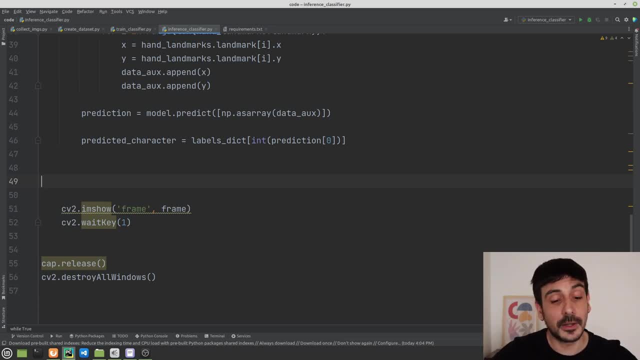 we have completed all the different steps. we have trained the classifier and now we are testing the classifier and everything seems perfect. we are testing this classifier with live data and everything seems perfect. so the only thing we're going to do now is to do call rectangle and we are going to input frame and then we are going to input. 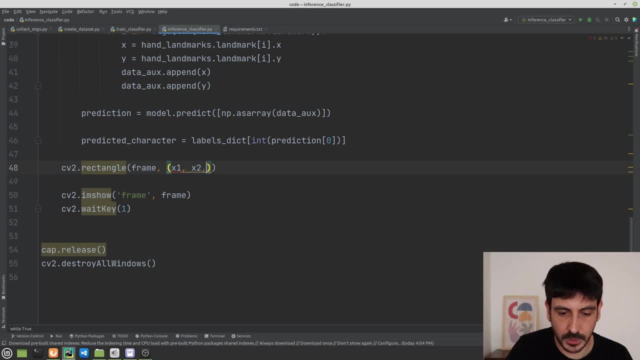 two values, which are x1 and x2, and then we are also going to input- sorry, this is y1 and this is x2- y2- a color which i'm going to define in black, because we have too many colors already in this picture, in this frame, with all the landmarks and so on, so i'm just going to set it in black. 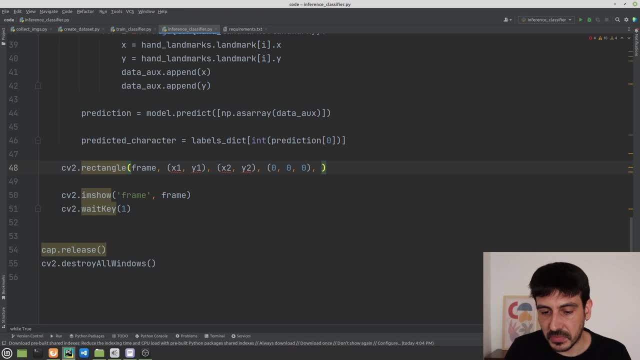 and then the thickness value, which will be, i don't know, four, something a4. and i'm just going to do this now and i'm going to, um, i'm going to define x1 and x and y1 and x2 and y2 in black. 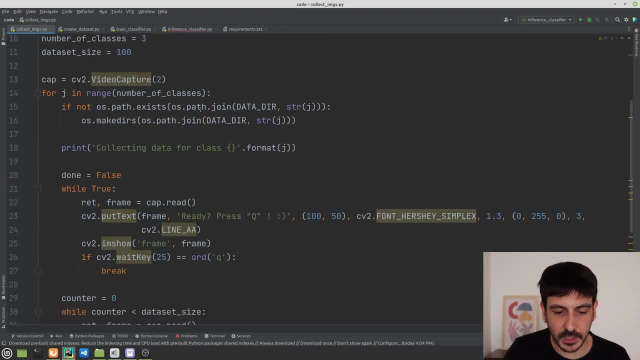 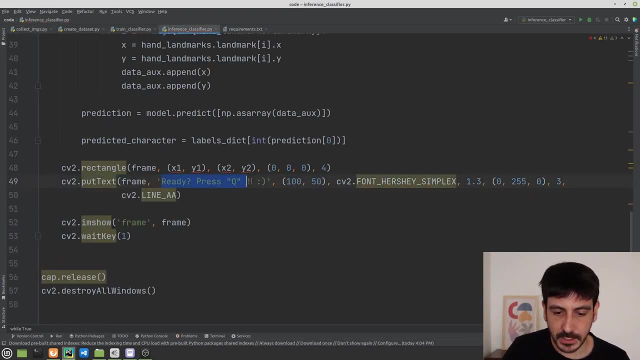 and then i'm just going to set the imagine a folder and then in a minute- but let's just continue for now- and i want to call put text and i have a put text here, so i'm just going to copy paste and i'm going to. 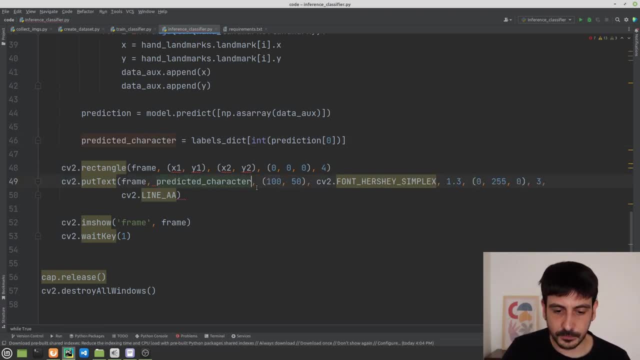 edit it with these values. this is going to be the class we are detecting, so it's exactly this. then this will be here. we should be super, super happy. This is only a detail to make a very pretty drawing, but everything is solved. everything is perfect. 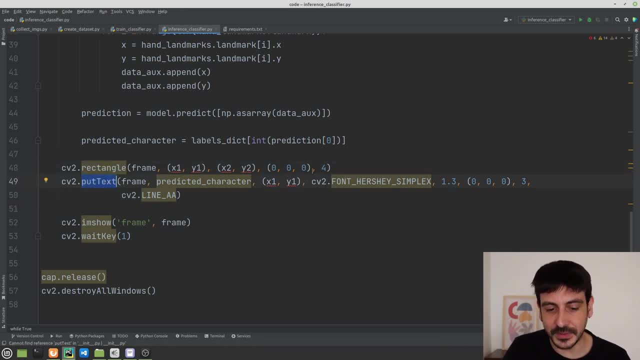 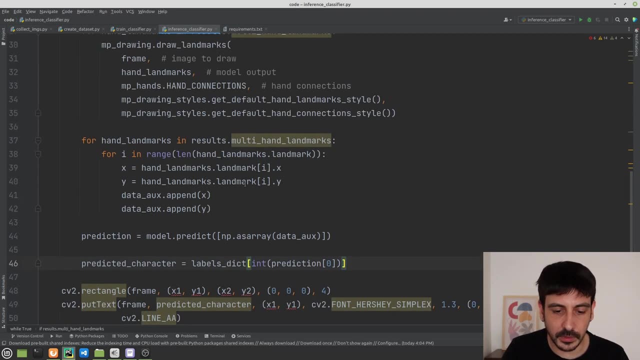 So we are drawing a rectangle and we also put in the text on top of this rectangle with the class we are predicting. And now we have to define these values. And in order to define these values, the way I'm going to do it, 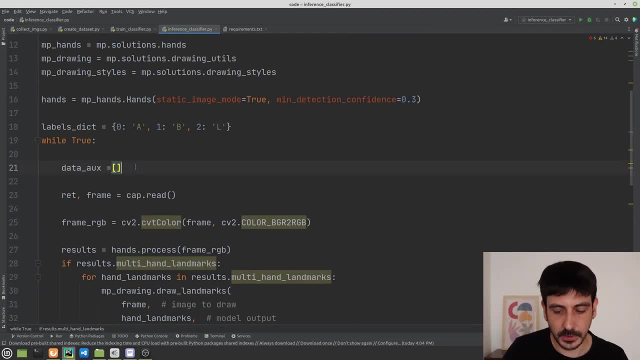 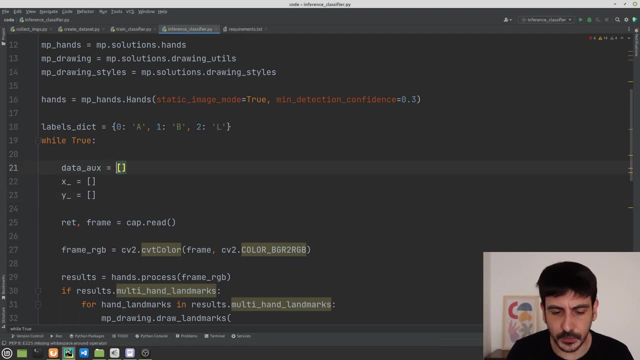 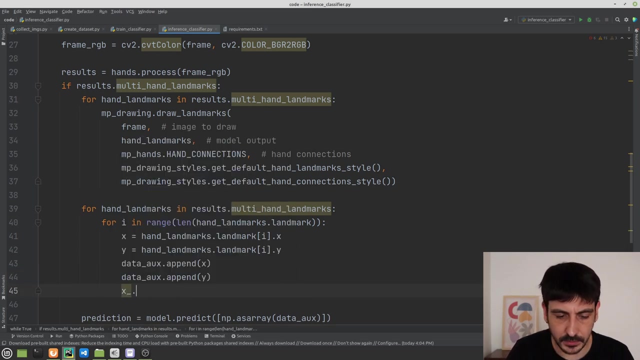 I'm going to define two additional arrays, which is here X and Y. I think this will be the easiest way to solve this problem. So I'm just: I have defined these two auxiliary arrays and I'm going to say X, dot, append X. 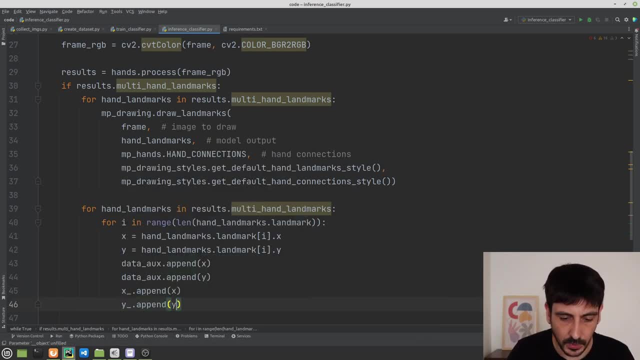 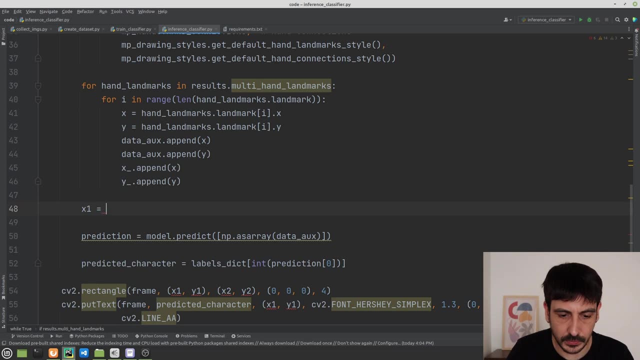 and then Y dot, append Y, And I'm going to say something like X1 equal to the minimum value of X, and then Y1 is exactly the same for Y, and then X2 and Y2 are the maximums. Remember, we are trying to get the corners. 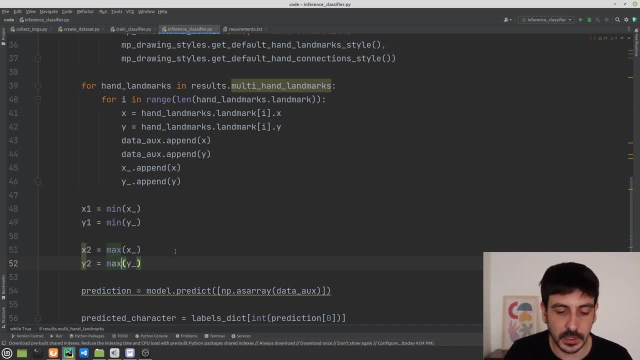 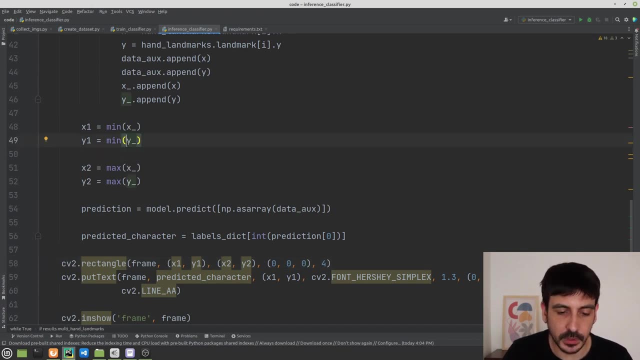 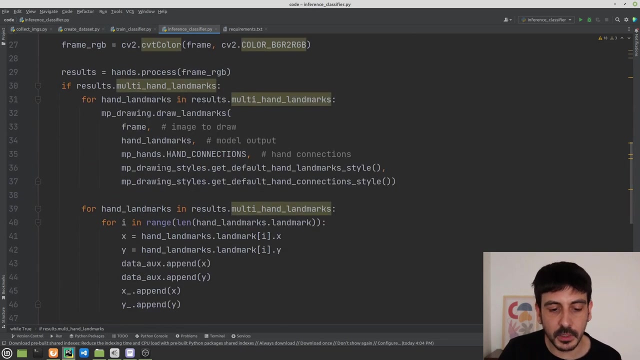 of the rectangle containing the hand, And we also, so we know exactly where to display this rectangle and this text. So we are going to do, but we need to do something else because, if you remember the values we were getting for the landmarks, everything is in a float. 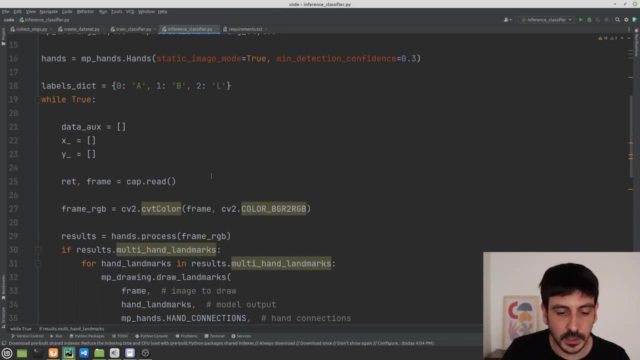 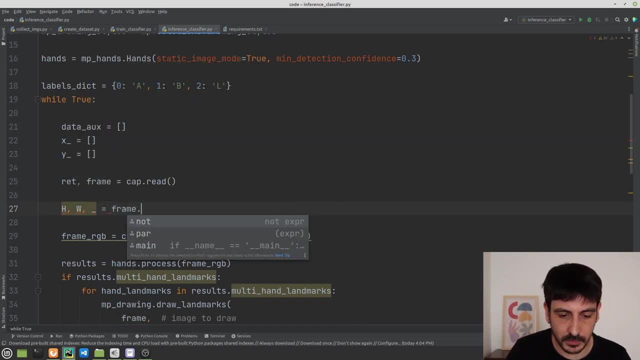 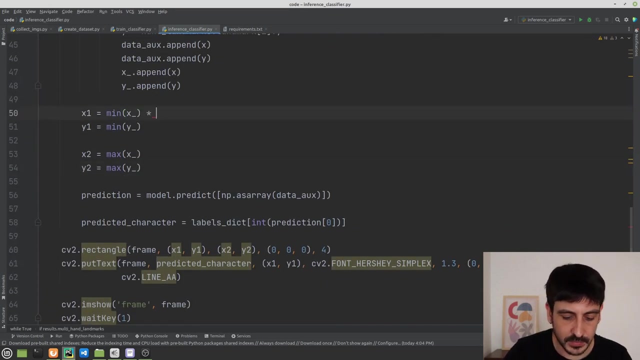 everything is float, So we need to convert it into an integer, And the way we're going to do it is by calling. we are going to get the frame shape, Everything's okay, And then we are just going to multiply this value times the width of our image. 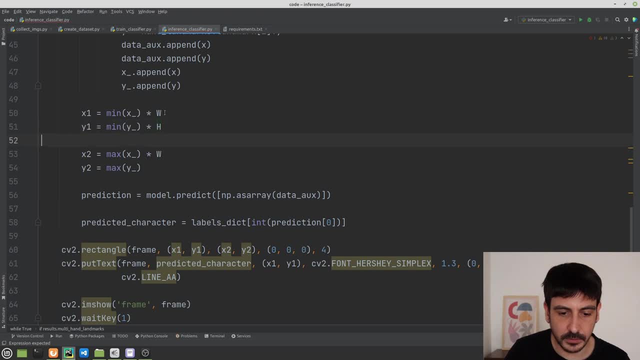 And we are multiplying the sort value times the height And we need to cast everything as an integer And this should be enough. Let's see how it performs. This is not necessary. Int, int, int. Okay, Okay, Let's see. let's see if it works. 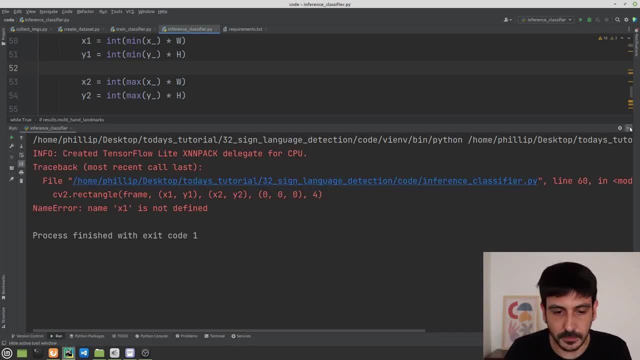 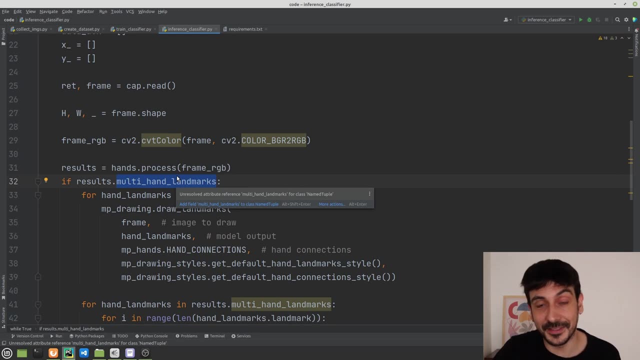 Or if we need to adjust something else. Okay, X1 is not defined. Okay, So the problem is that if we are not detecting any hands, right, if there's not any hand in the frame, then we never execute this loop. 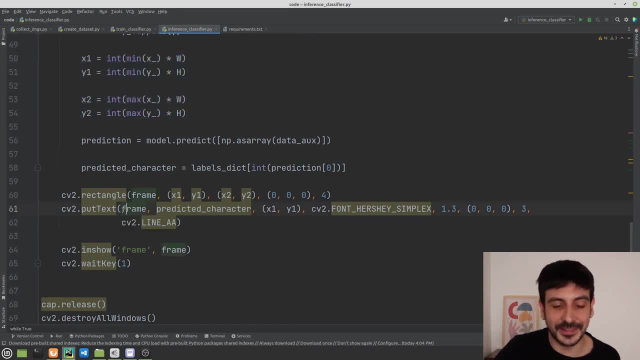 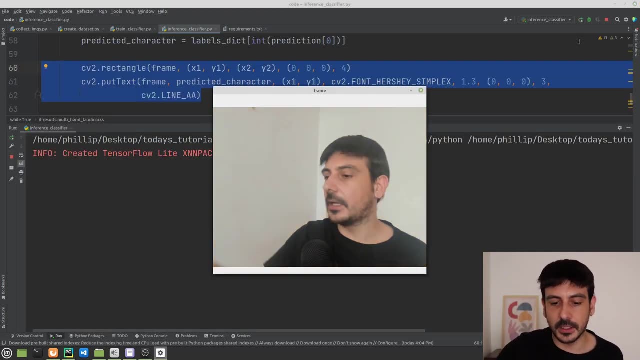 We never define these variables and we cannot draw the rectangle and the text in the location we specify, So doing something like this should be enough. Now let's execute it again, And I'm just going to do an A And you can see that I'm classifying the A.